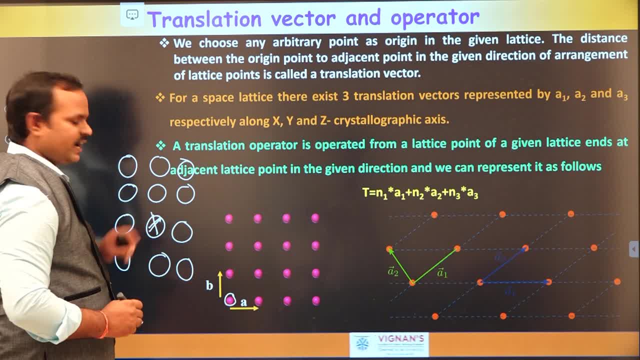 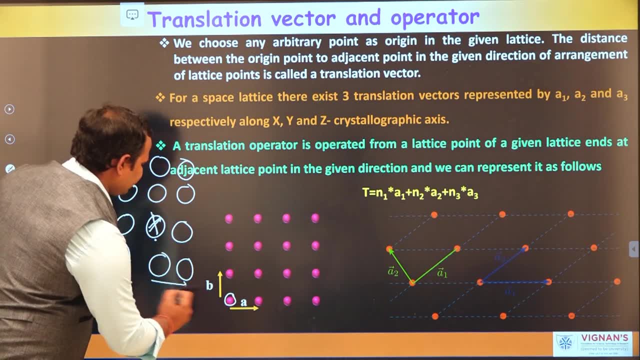 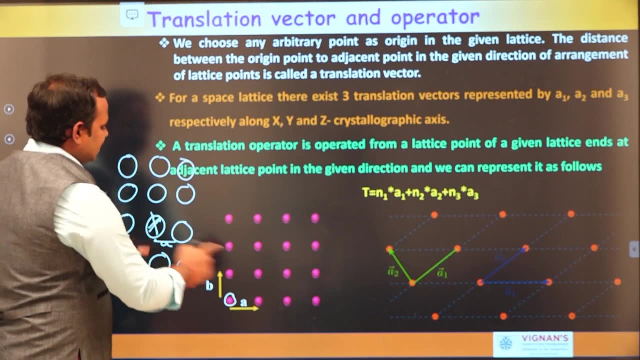 So this is a point that I am placing for this corresponding atom. Now let us find in a given direction. This is the direction I am considering: The distance between the two atoms. This is the A. Now let us place another point in the space, at a distance. 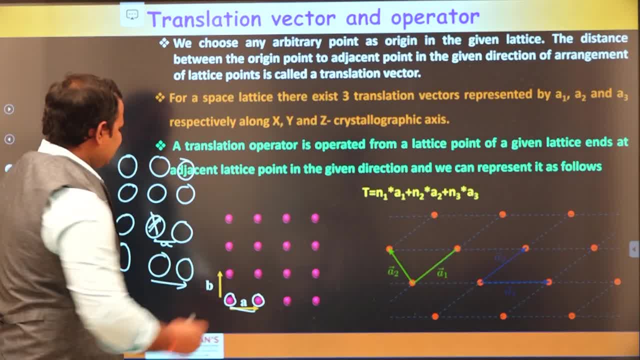 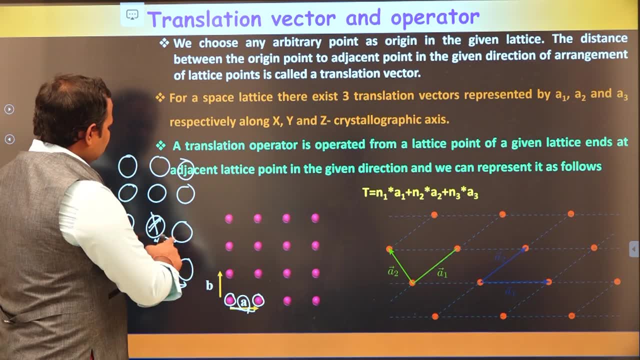 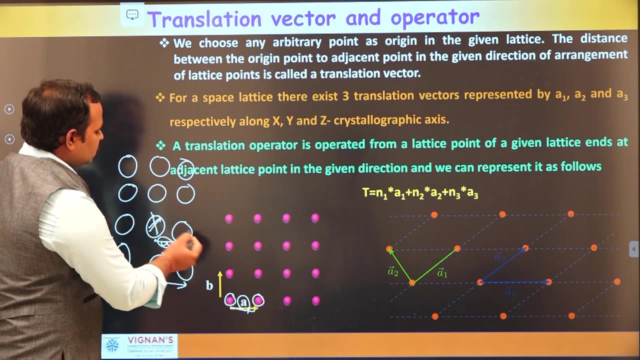 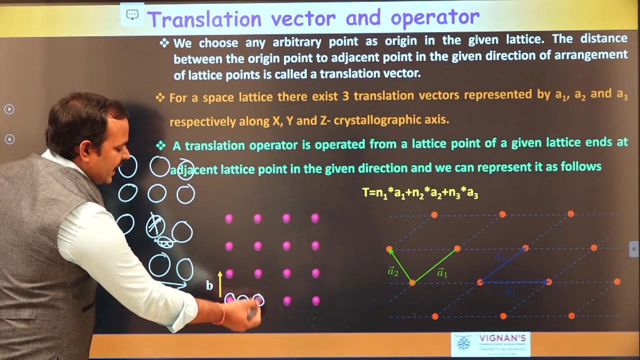 The distance between the two atoms is the distance between A and A from the origin. That means this is the translational vector in the space. Now, since in the crystal the atoms are arranged regularly periodically in three dimensions, So in this dimension the atoms are arranged regularly continuously. 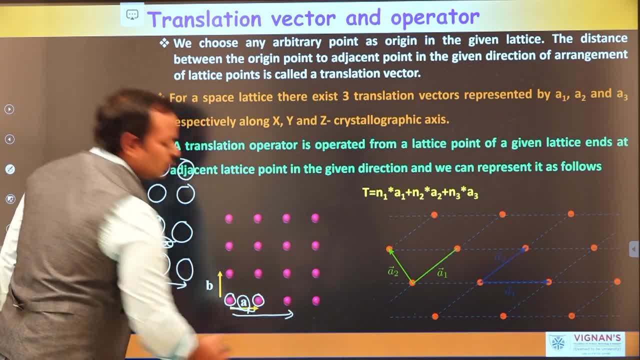 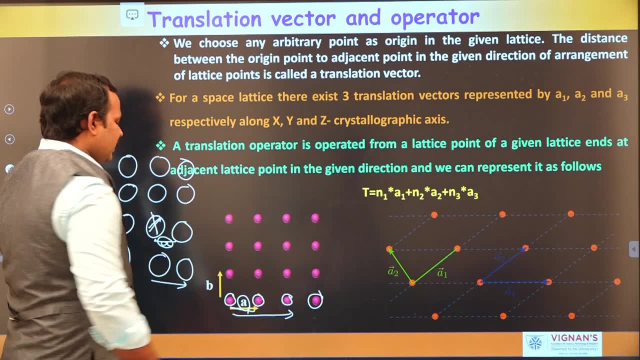 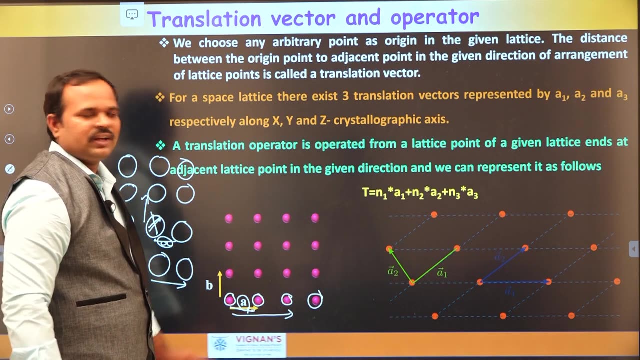 So now, if we repeat the atoms with the distance A in the x direction, we get some more points. So this is another point. This is another point. Similarly, let's find another direction, And this is called a translational vector in the space. 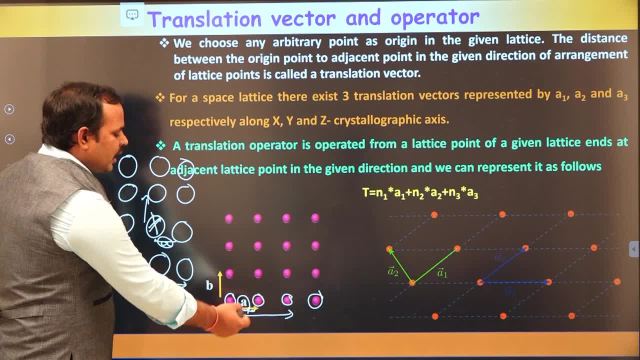 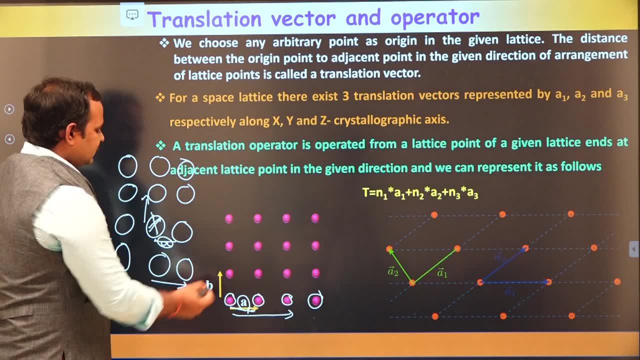 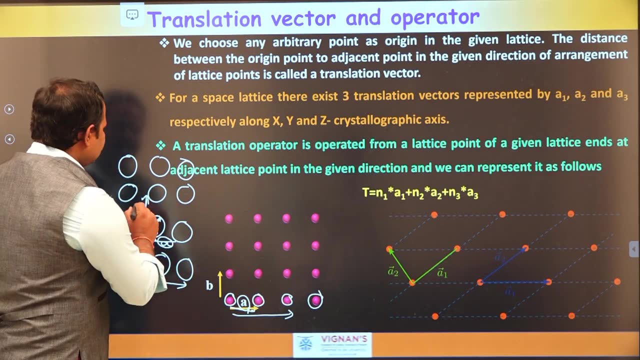 Now, by using this translational vector, we operate this translational vector in the space to get other points in the lattice. Now let us consider another direction in the real crystal. This is the y direction I am considering And the distance between the two atoms is. the successive atoms in this y direction is B. 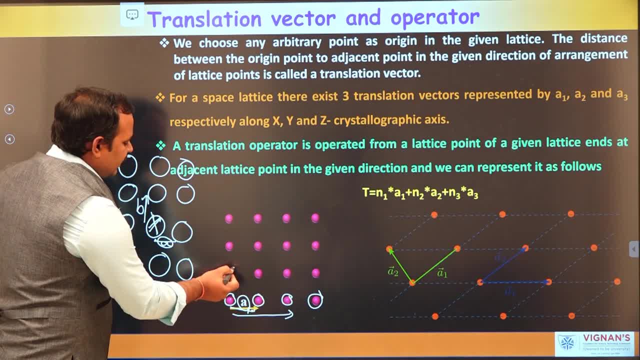 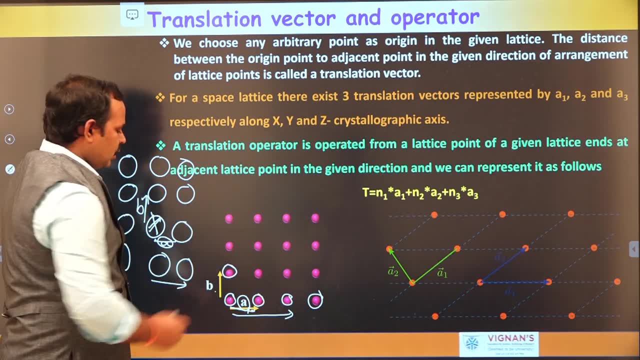 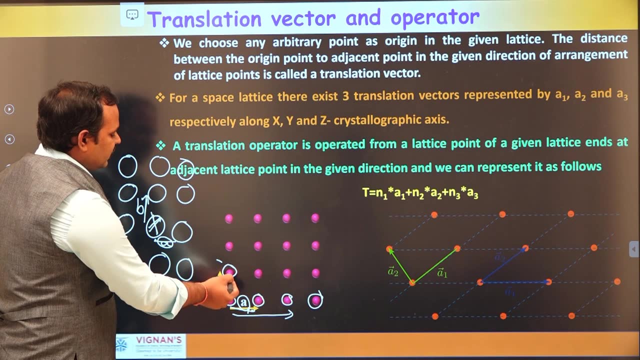 Now. so let's place another atom in the y direction in the space, at a distance: B Now we have kept B. Now this is the translational vector in this direction. Now repeat this translational vector in the y direction by using operator. 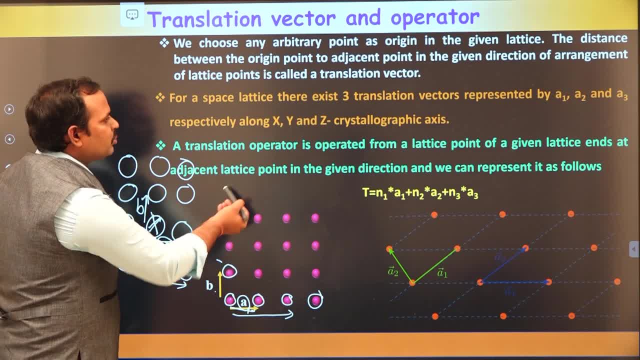 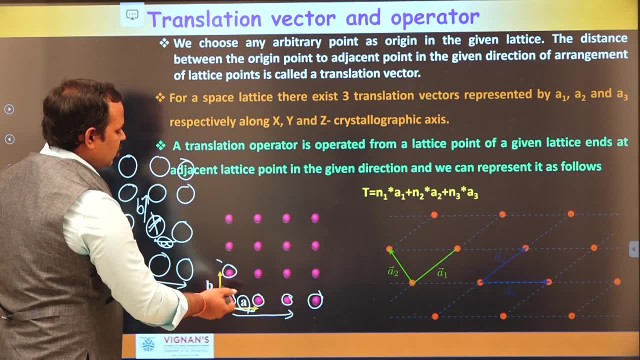 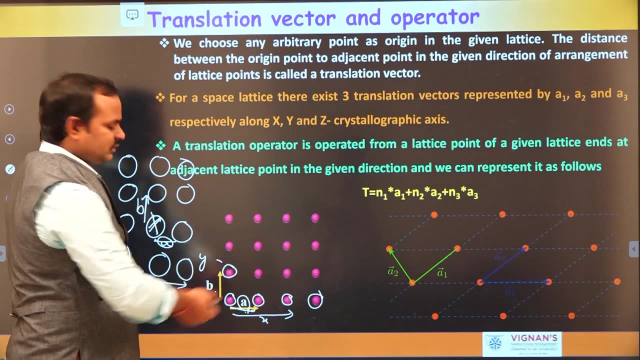 That means you repeat this B to get other points in this direction. Now let us operate this translational operator on translational vector A and B in both x and y directions, with a periodicity A and B, So we get all other points. 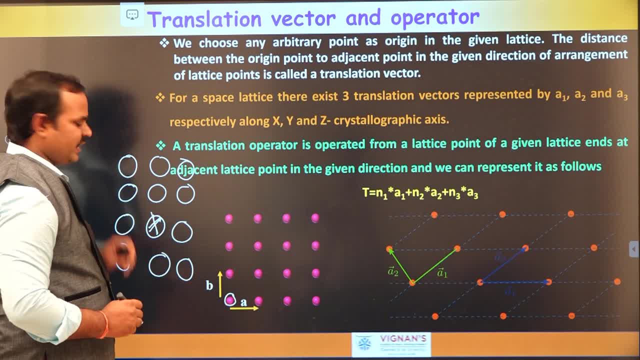 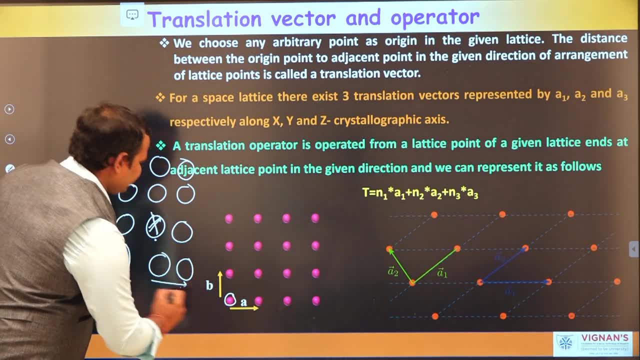 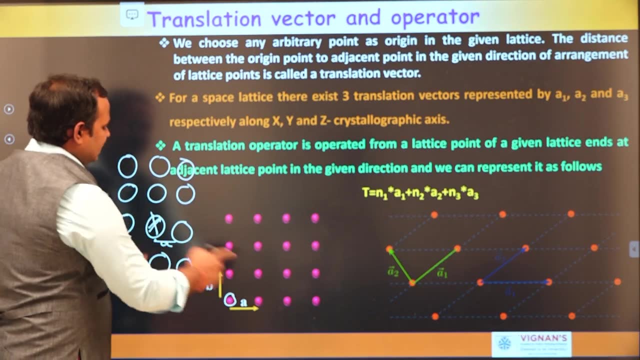 So this is the point that I am placing for this corresponding atom. Now let us find in a given direction. This is the direction I am considering- The distance between the two atoms. This is the A. Now let us place another point in the space at a distance A. 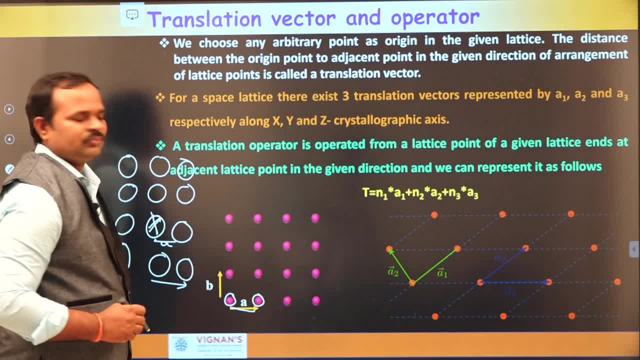 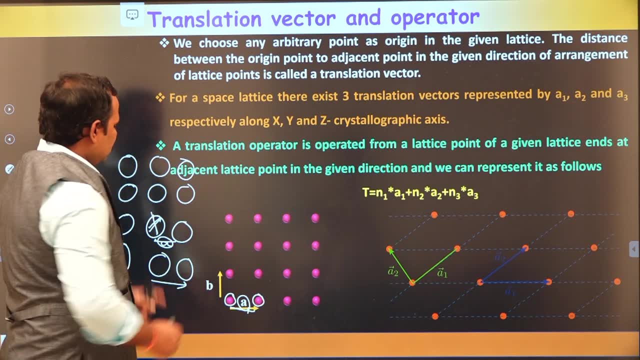 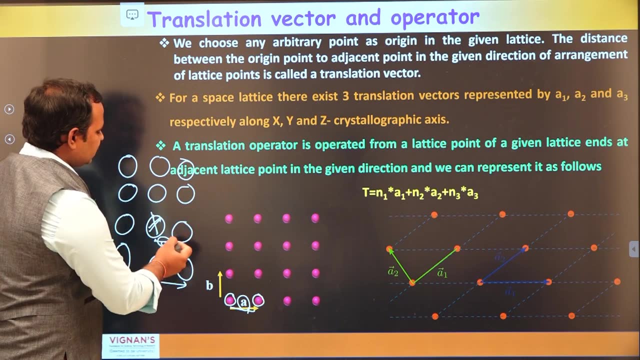 This is the distance A from the origin. That means this is the translational vector in the space. Now, since the crystal is in the crystal, the atoms are arranged regularly, periodically, in three dimensions. So in this dimension the atoms are arranged regularly, continuously. 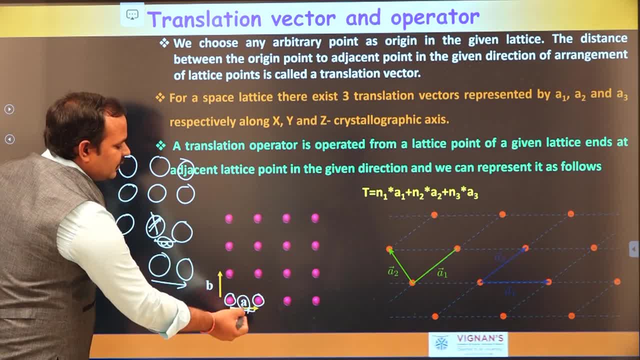 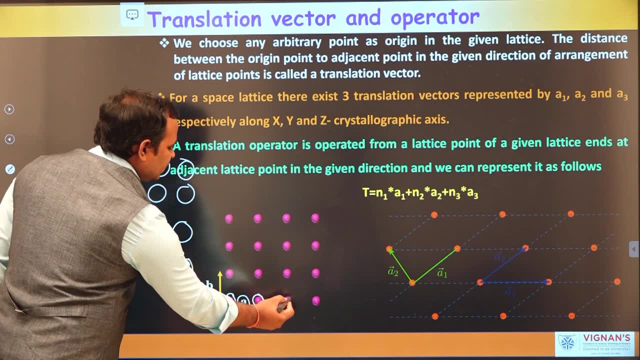 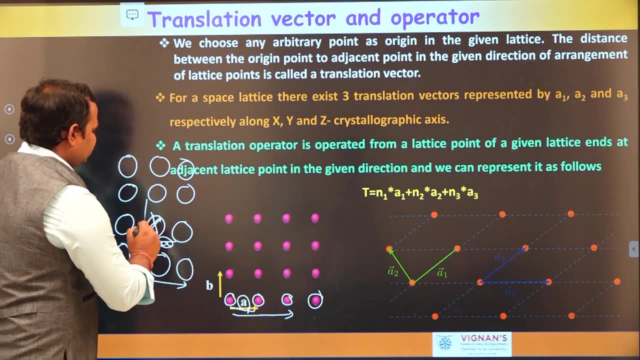 So now, if we repeat the atoms with the distance A in the x direction, we get, We get, We get some more points. So this is another point, This is another point. Similarly, let's find another direction, And this is called a translational vector in the space. 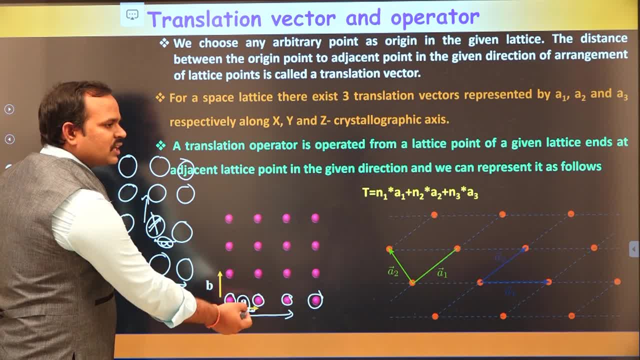 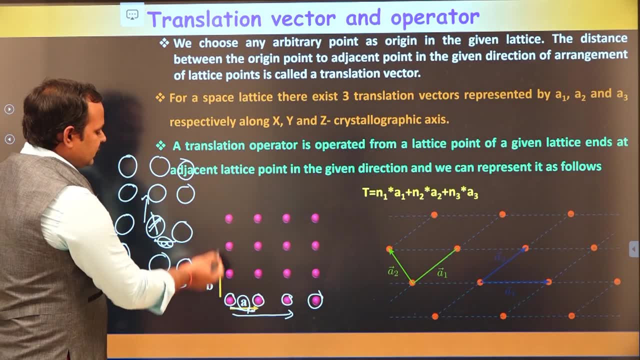 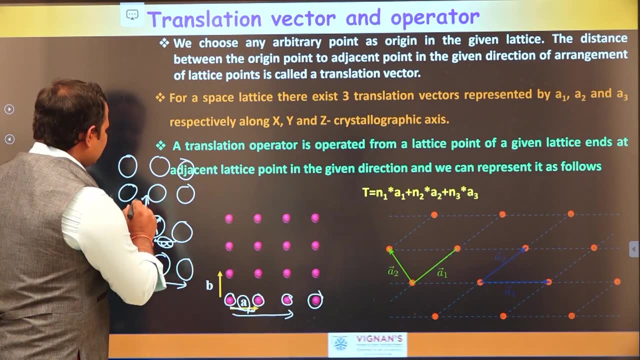 Now, by using this translational vector, we operate this translational vector in the space to get other points in the lattice. Now let us consider another direction in the real crystal. This is the y direction I am considering And the distance between the two atoms is. the successive atoms in this y direction is B. 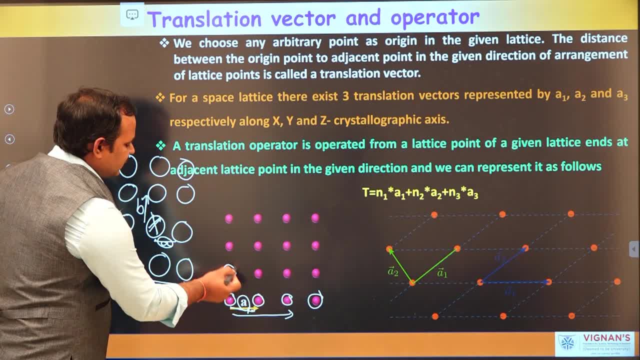 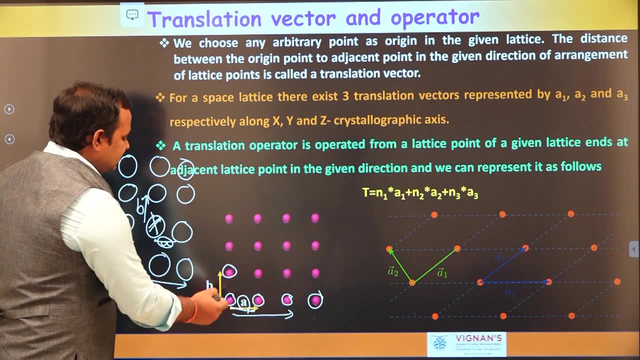 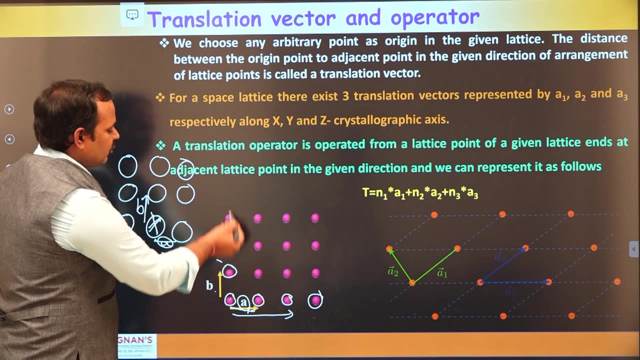 Now. so let's place another atom in the y direction in the space, at a distance: B Now we have kept B. Now this is the translational vector in this direction. Now repeat this translational vector in the y direction by using operator. 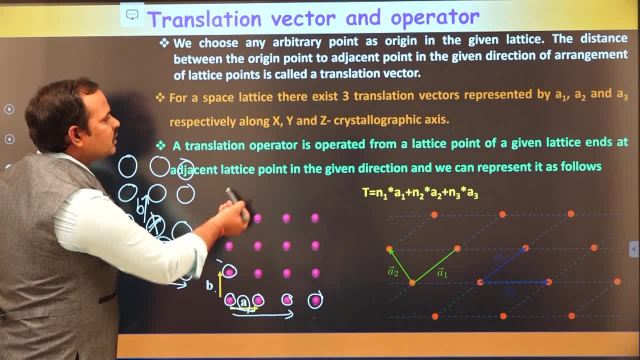 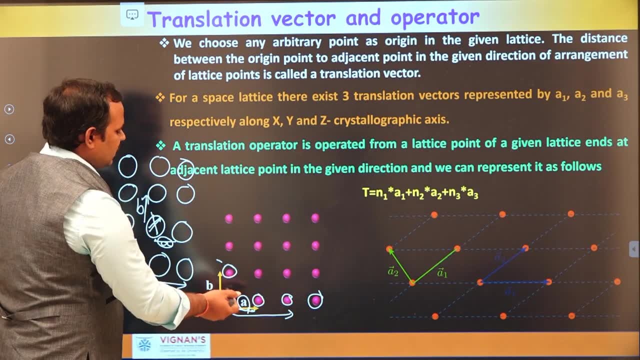 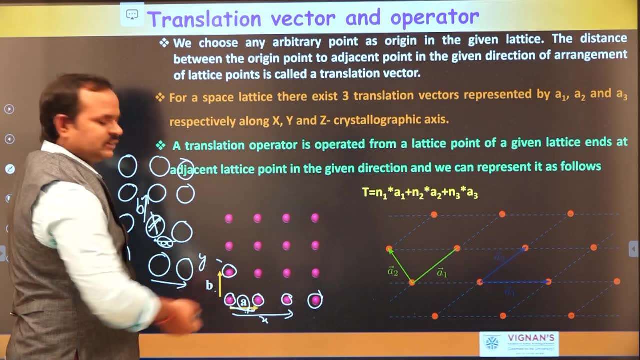 That means you repeat this B to get other points in this direction. Now let us operate this translational operator on translational vector A and B in both x and y directions, with a periodicity A and B, So we get all other points. 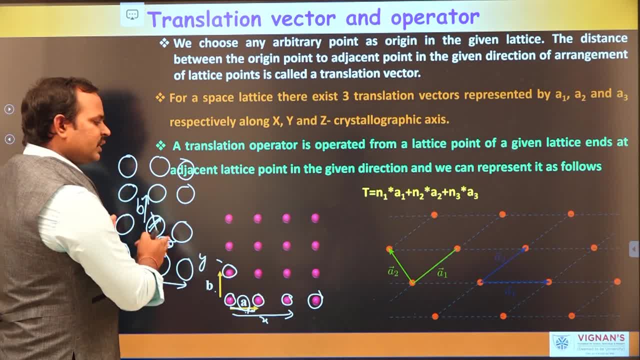 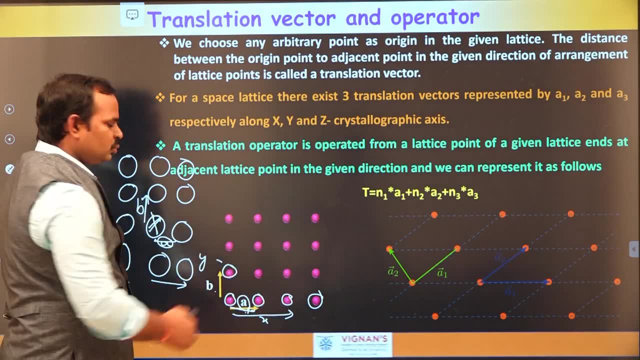 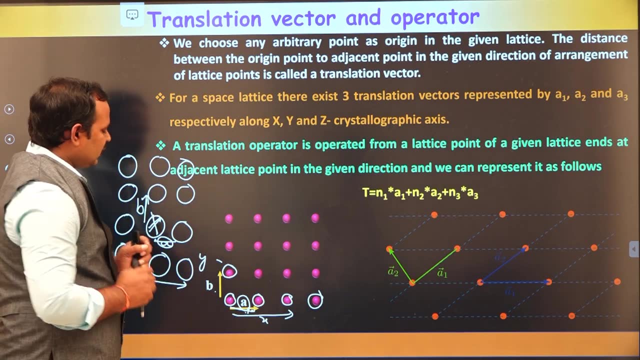 In this way, we can visualize a two-dimensional crystal in a space by using geometry. Now, all these are points which represent the atoms in the real crystal. Now the question is: why only in this direction? Why can't we visualize another direction? 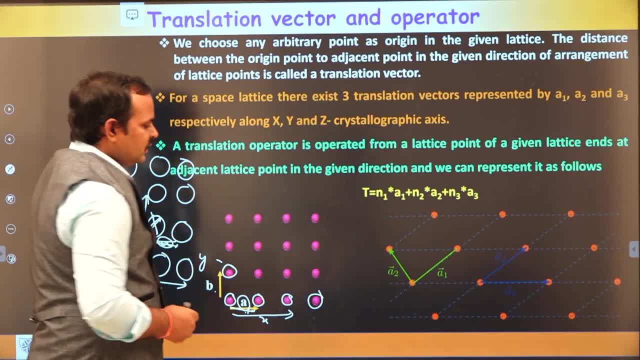 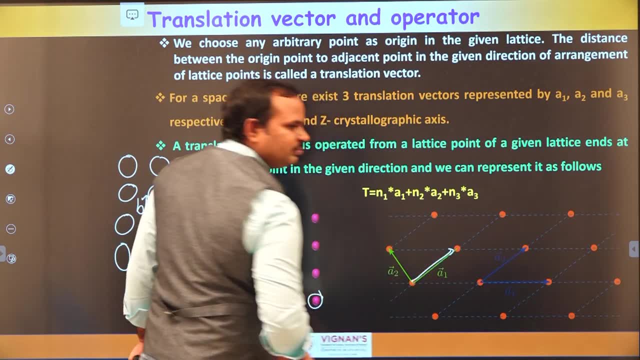 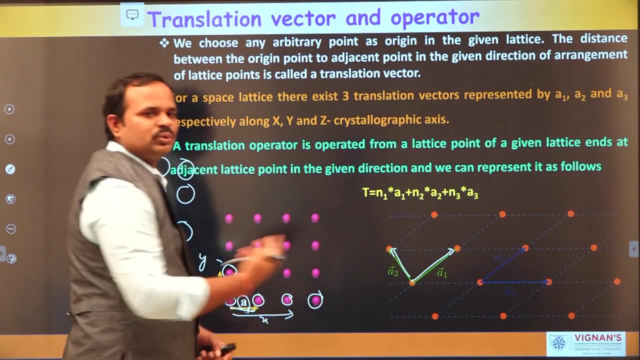 Yes, we can even consider another direction. For example, let us consider: this is another crystal. We can also consider the direction. This is one direction- and can construct the lattice points. This is another direction. This is a two-dimensional, So we only have two translational vectors. 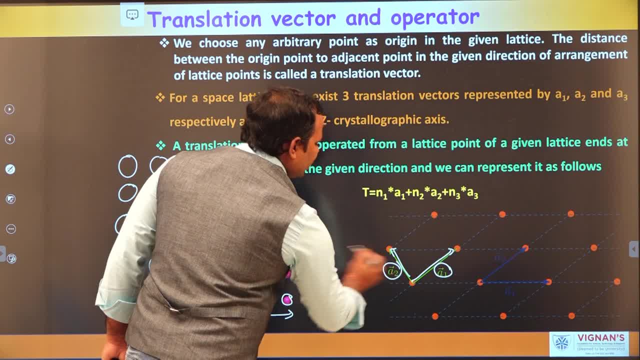 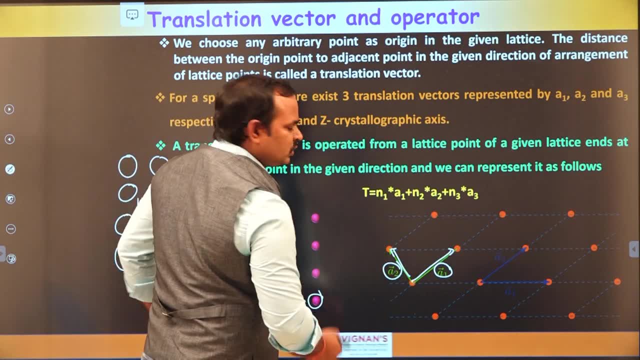 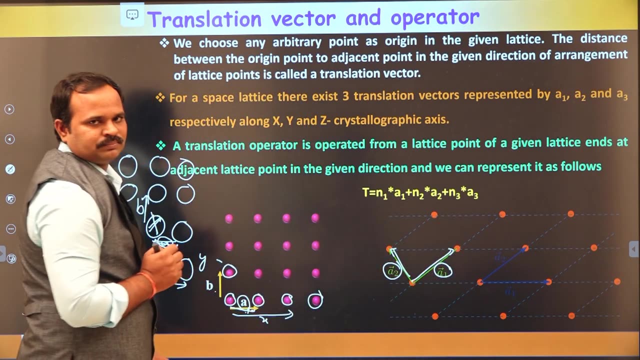 So A1 is in one direction, A2 is in one direction. Previously we have considered the x and y direction, But here we are considering random directions. Now with these translational vectors we can repeat in two dimensions to get a total lattice. 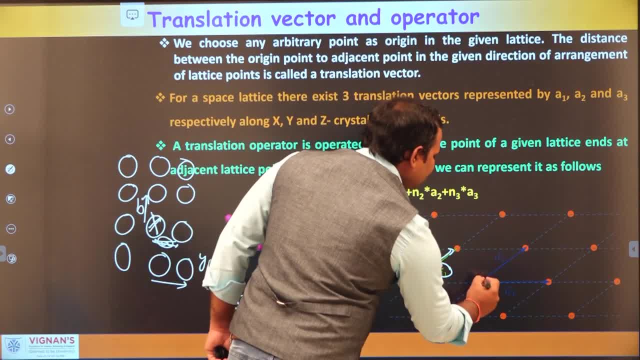 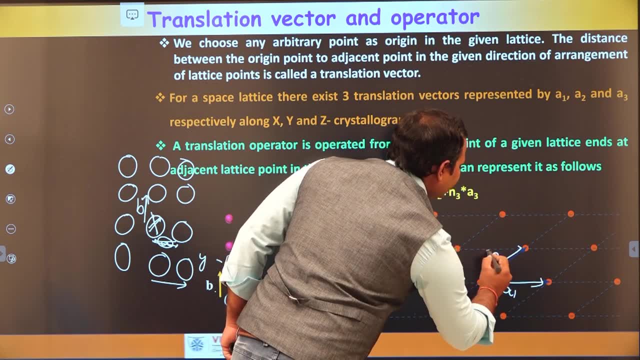 We don't need to take only these two. We can also take another direction. For example, this is a one direction, This is another direction. So let's consider: this is A1.. This is A2.. This is a translational vector. 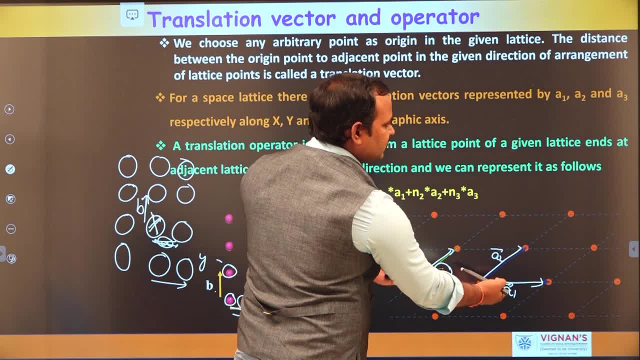 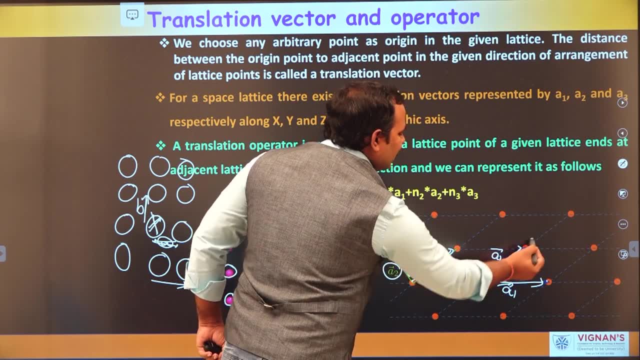 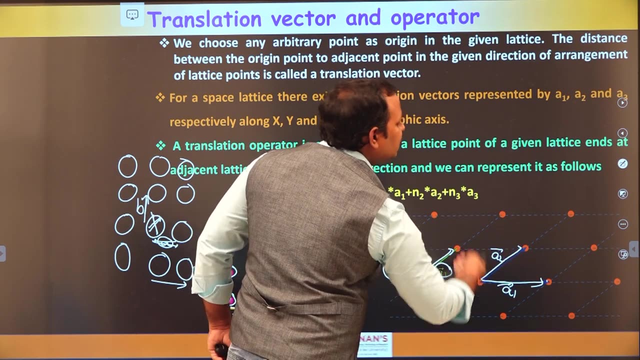 Now, even in this way also, we can consider: this is the origin point, This is the distance between the two successive points in this direction, This is the distance between the two successive points in another direction. Now, with these two translational vectors, we can again construct the space lattice similar to the crystal structure. 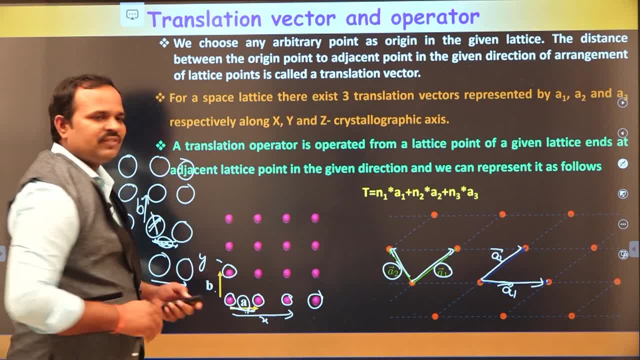 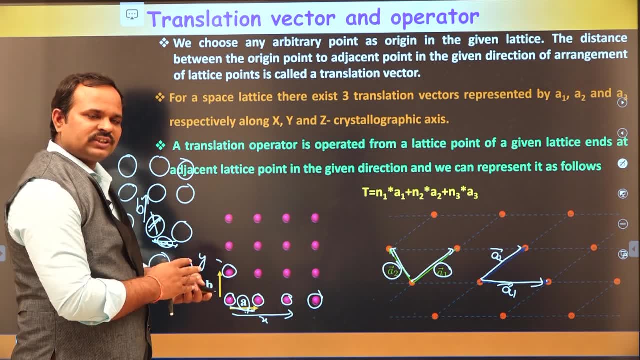 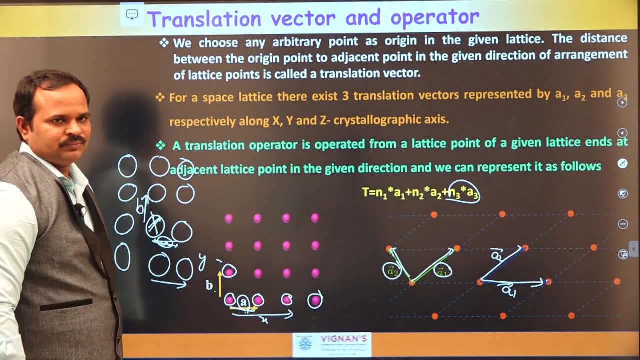 So this is by using a translational vector and a translational operator And, for example, if we are considering a three-dimensional crystal, then we also have a third translational operator, A3.. So the translational operator will work like this way. 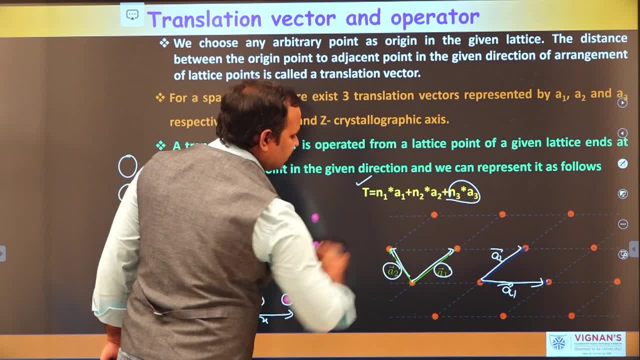 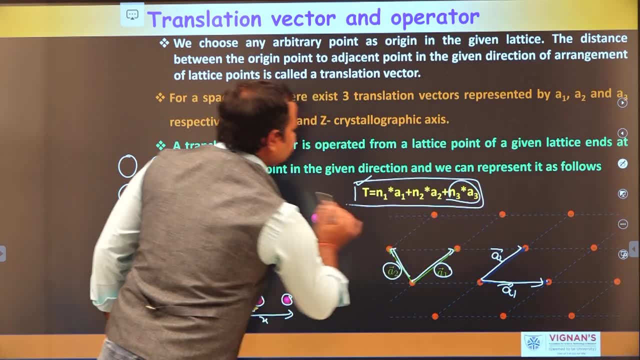 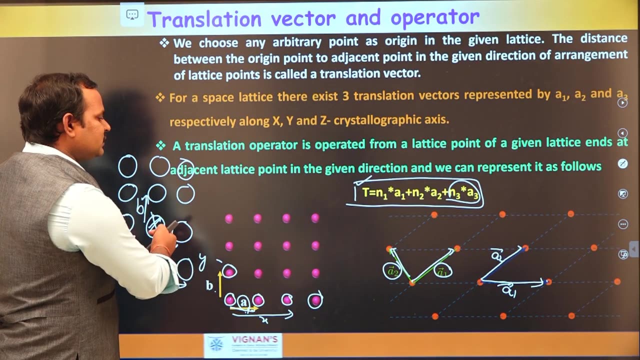 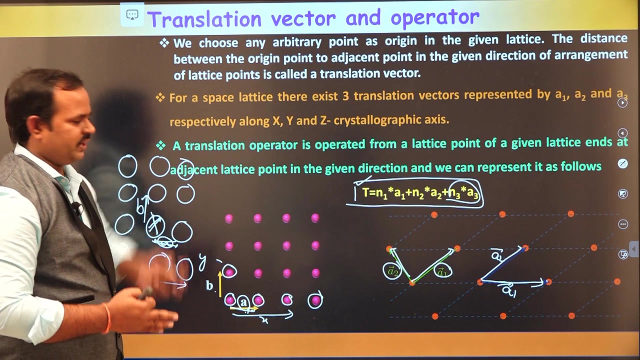 T is equal to N1A1 plus N2A2 plus N3A3.. So we can get any point position by using this, This operator. So now, by the end of this, we understand that we can construct a lattice in a space by using a translational vector and operator. 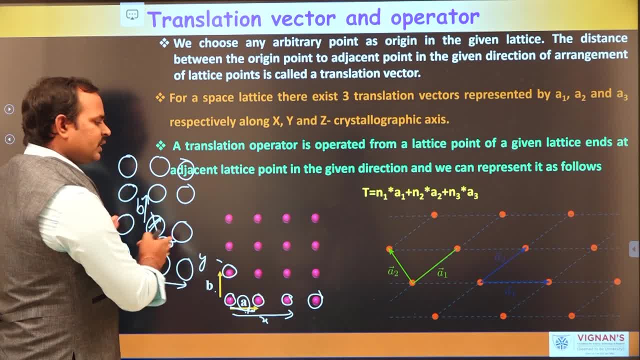 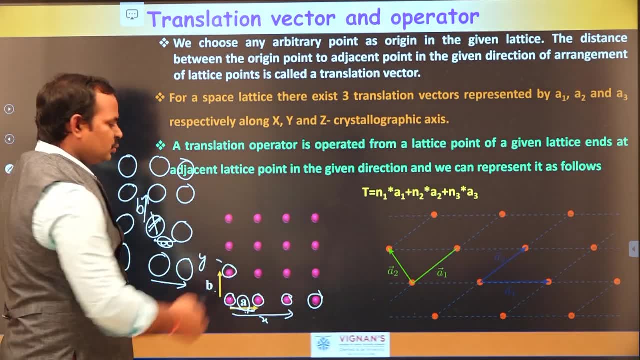 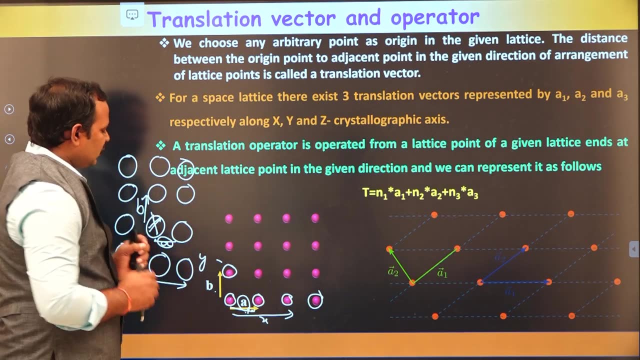 In this way, we can visualize a two-dimensional crystal in a space by using geometry. Now, all these are the points which represent the atoms in the real crystal. Now the question is: why only in this direction? Why can't we visualize another direction? 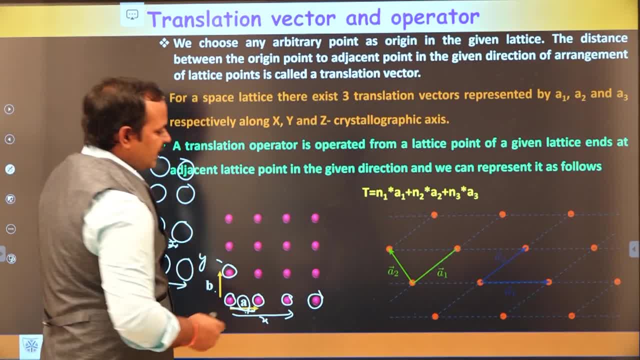 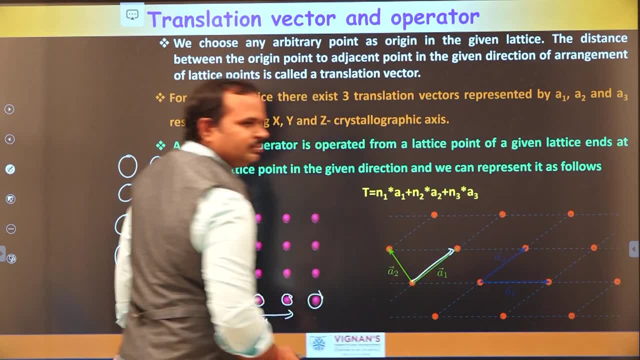 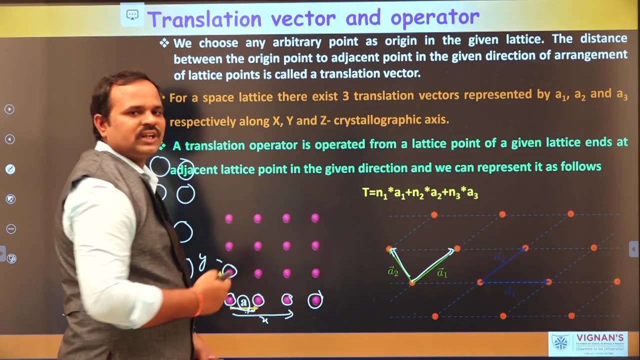 Yes, we can even consider another direction. For example, let us consider: this is another crystal. We can also consider the direction. This is one direction- and can construct the lattice points. This is another direction. This is a two-dimensional, so we only have two translational vectors. 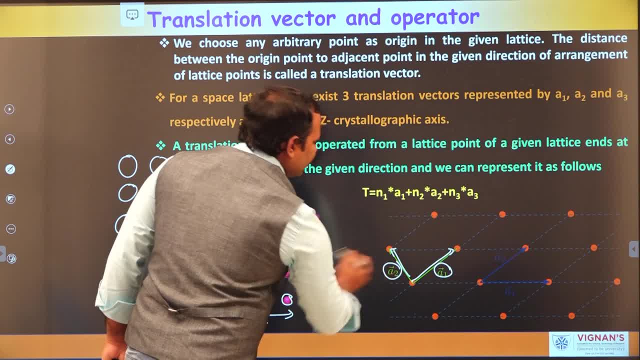 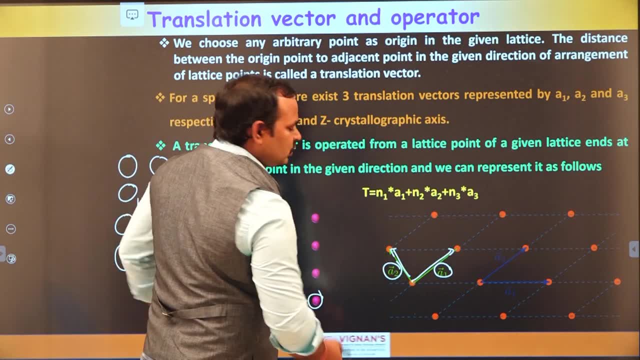 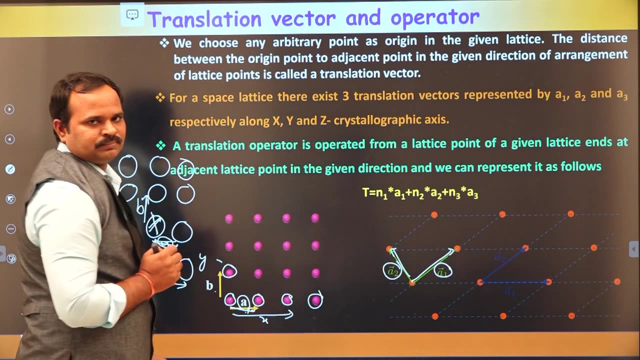 So this is: A1 is in one direction, A2 is in one direction. Previously we have considered the x and y direction, but here we are considering random directions. Now with these translational vectors we can repeat in two dimensions to get a total lattice. 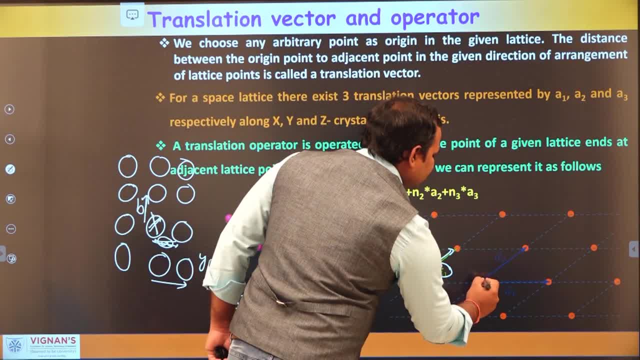 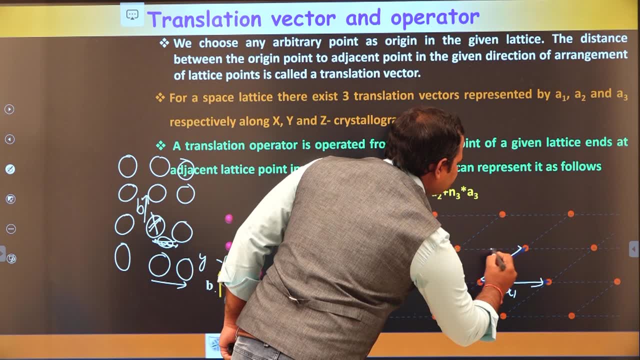 We don't need to take only these two. We can also take another directions. For example, this is a one direction, This is another direction. So let's consider: this is A1.. This is A2, is a translational vector. 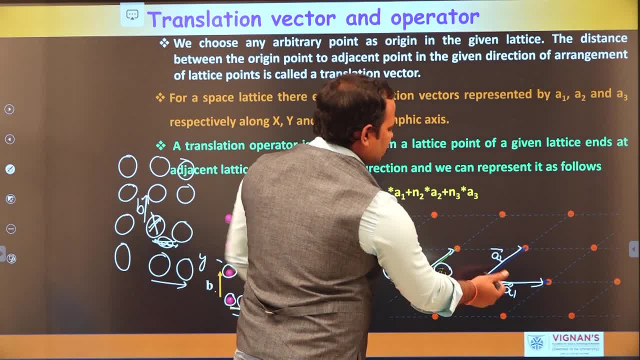 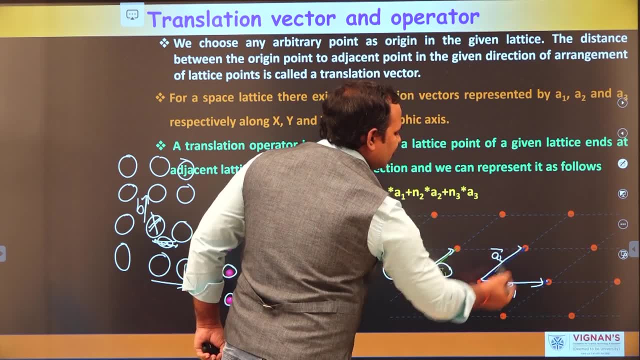 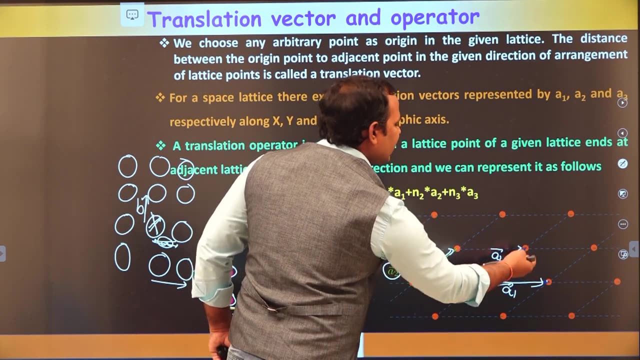 Now, even in this way also, we can consider: this is the origin point, This is the distance between the two successive points in this direction, This is the distance between the two successive points in another direction. Now, with these two translational vectors, we can again construct the space lattice similar to the crystal structure. 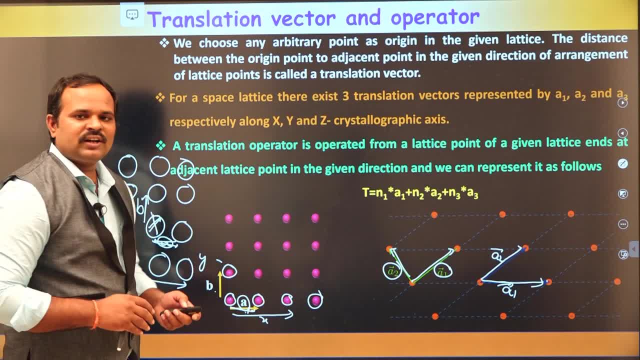 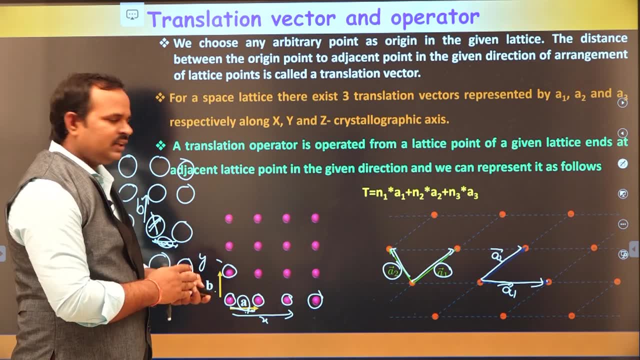 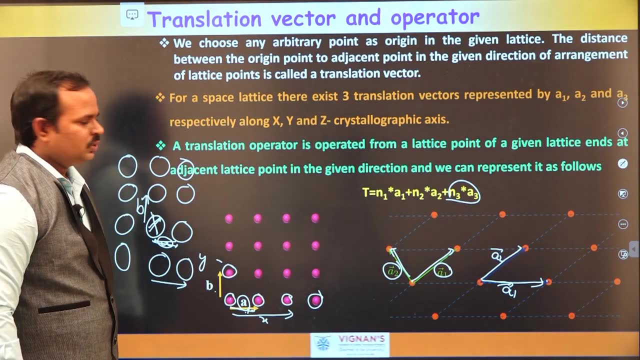 So this is by using geometry, This is by using a translational vector and a translational operator And, for example, if we are considering a three-dimensional crystal, then we also have a third translational operator, A3.. So the translational operator will work like this way: 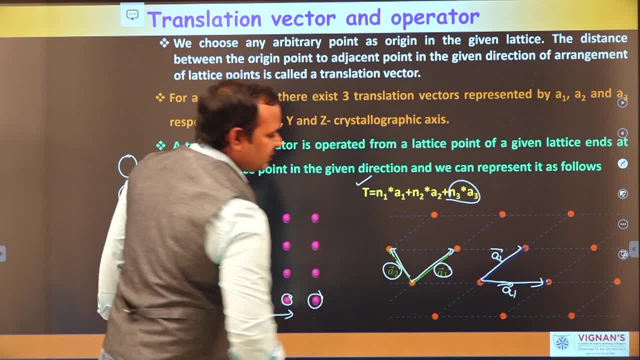 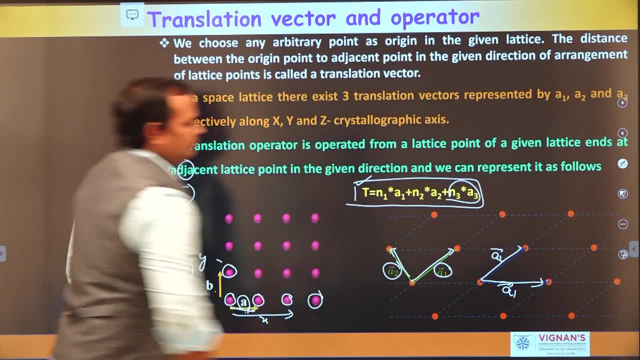 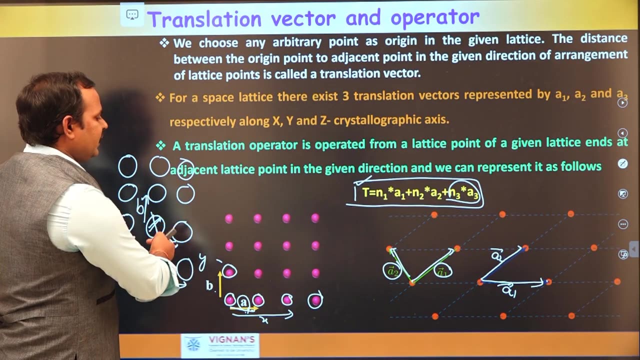 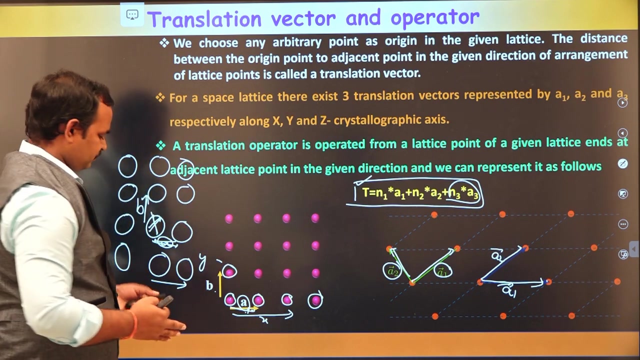 T is equal to N1, A1 plus N2, A2 plus N3, A3. So we can get any point position by using this operator. So now, by the end of this, we understand that we can construct a lattice in a space by using a translational vector and operator. 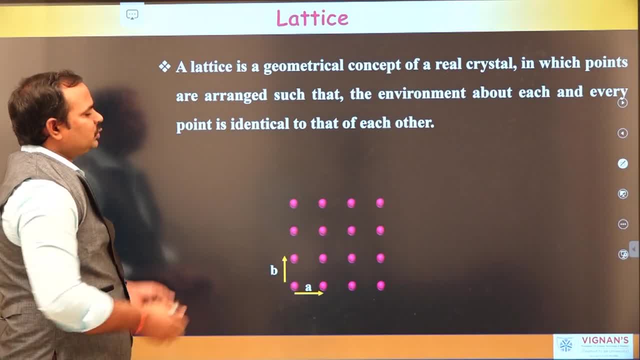 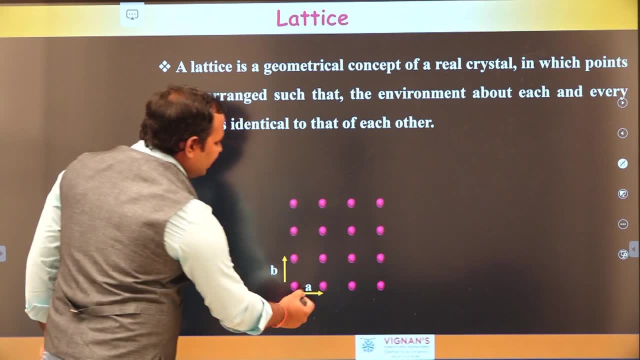 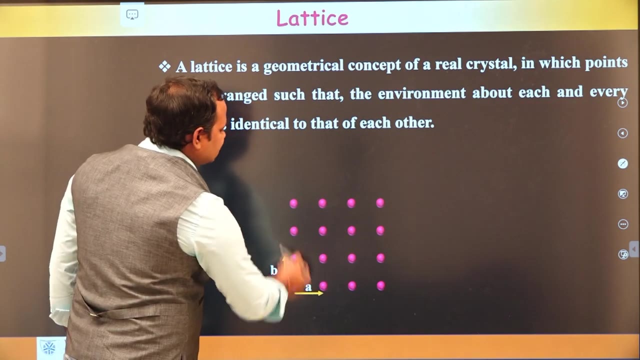 So a lattice means So. a lattice is a geometrical concept of real crystal in which the points are arranged such that the environment about each and every point is same. So that means what is the meaning is So, for example, this is the lattice that we constructed for some real crystal. 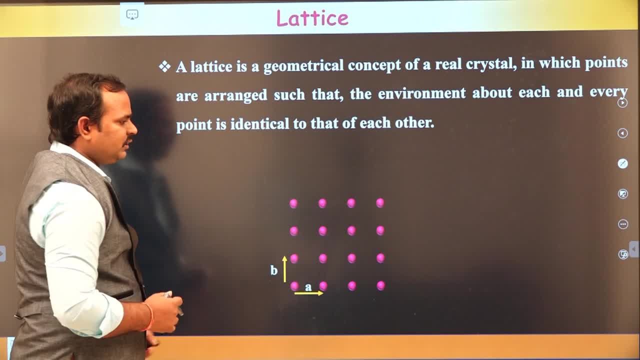 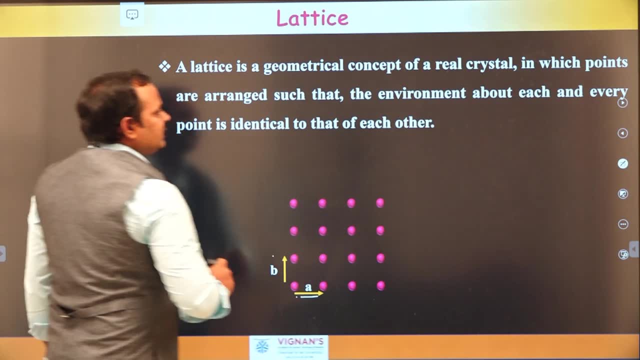 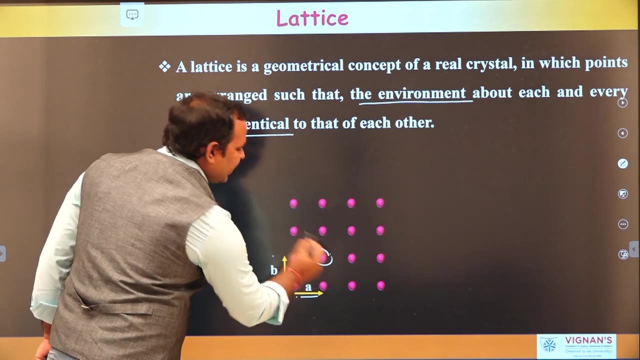 This is the lattice we constructed for some real crystal. Here the translational vectors are A and B And here the condition is the environment about. each and every point is identical. That means, for example: let us consider: this is the point I am taking. 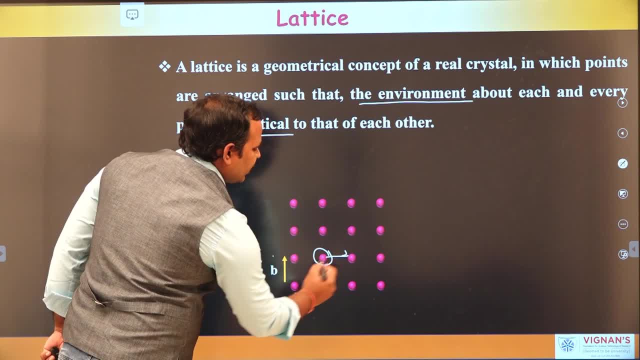 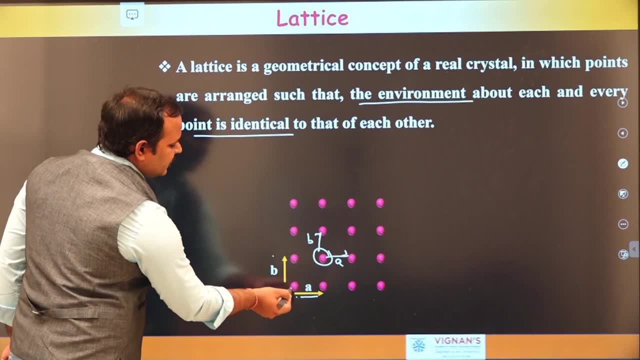 And let us see the distance between the two successive points in this direction. It is A and the distance between the two successive points in this direction is B, Which is similar. For example, if you take this is the same At the A distance. we have another point. 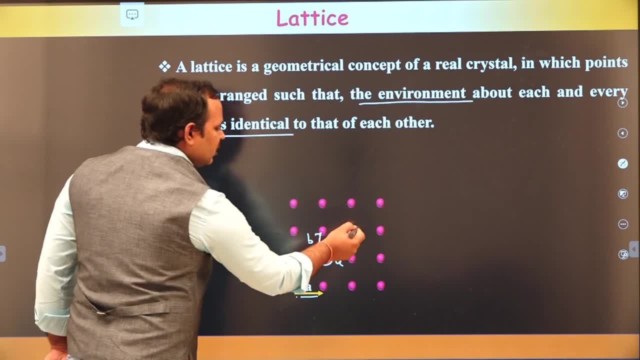 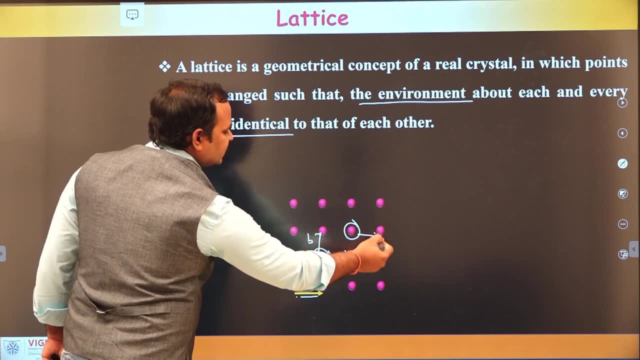 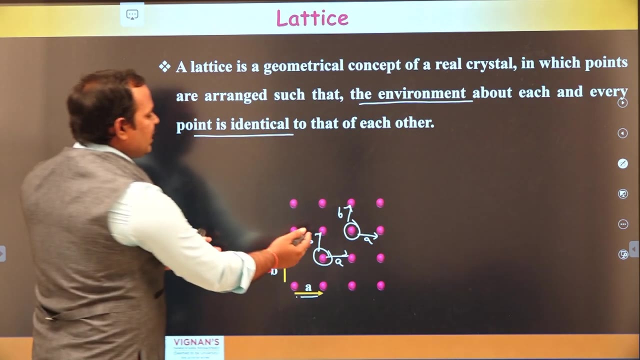 And the B distance. we have another point in this direction. Similarly, we can also take any atom. The distance between the two successive atoms in the x direction is A and the distance between the two successive atoms in the y direction is B. That means the environment about each and every atom is identical to B. 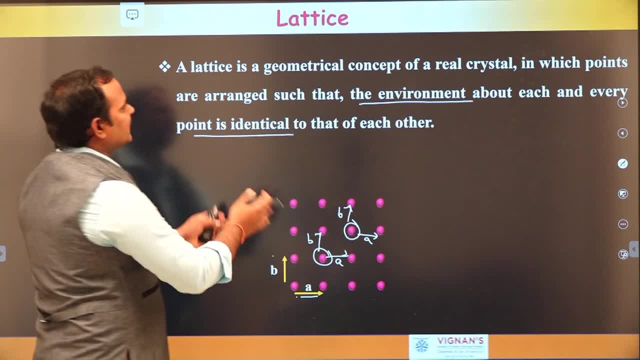 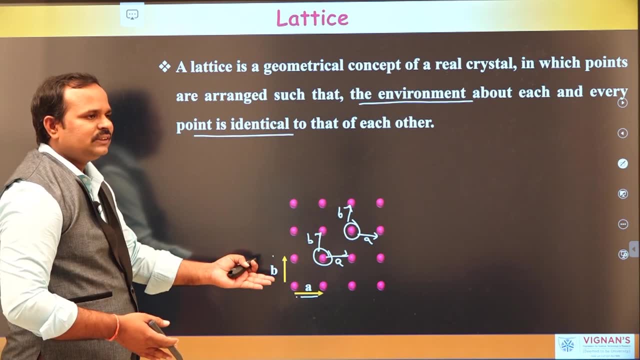 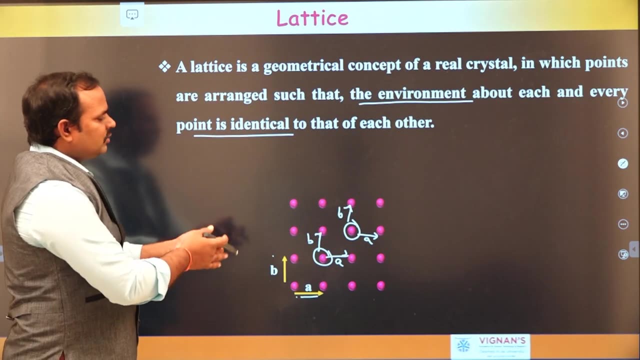 identical to each other. So this is called a lattice, This lattice. this is only a points. Now, these points, if you replace with the atoms in the crystal, we get a total crystal structure. You will get more clear as you go on. So a 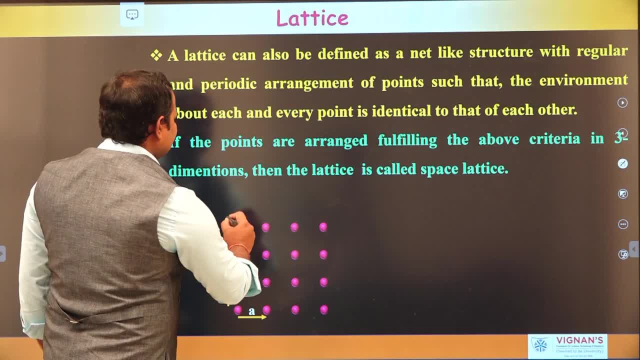 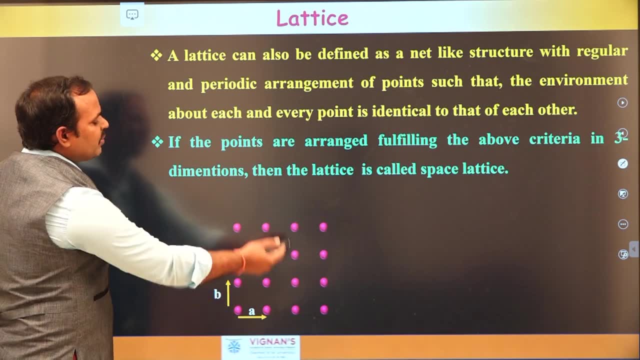 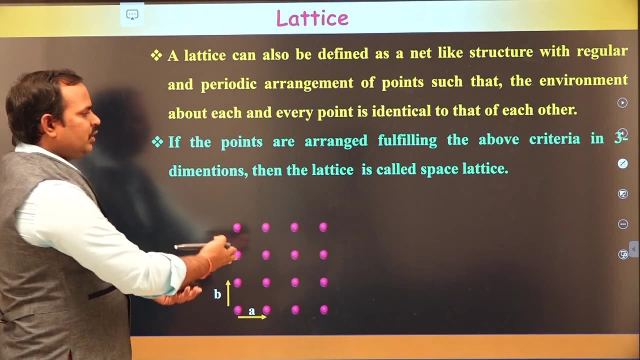 lattice can also be said as a net like structure, with regular, periodic arrangement of points in space, such that the environment about each and every point is identical. For example, if you replace these atoms, if you continue, I mean if you fulfill these atoms in three dimensions, we get a space. 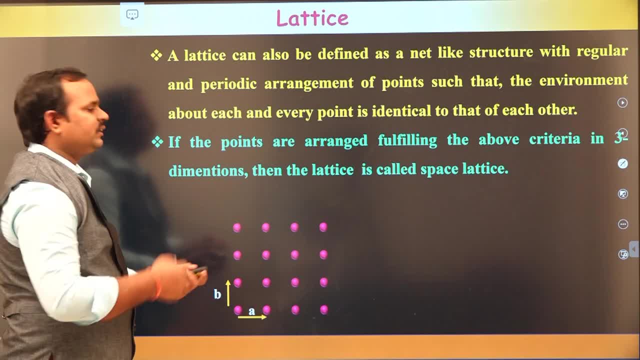 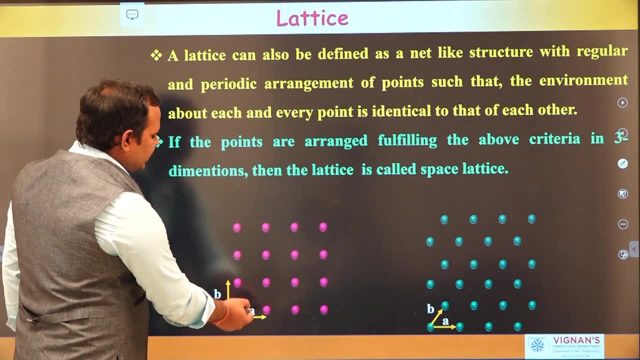 lattice. This is a two-dimensional lattice. We also get a three-dimensional lattice that's called a space lattice. So, as I told you, the lattice no need to be only having these two. We also have a translational vectors in another direction, In this case. 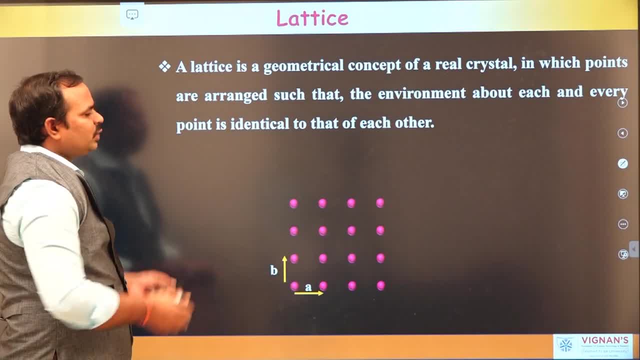 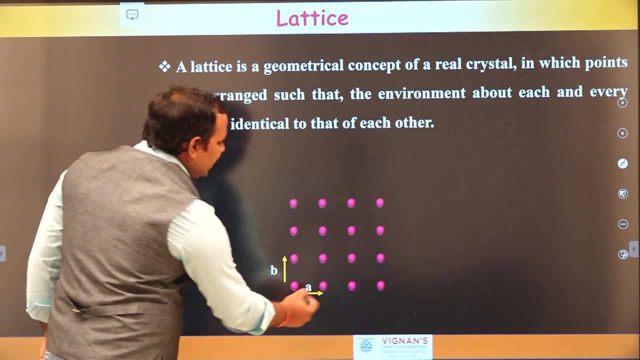 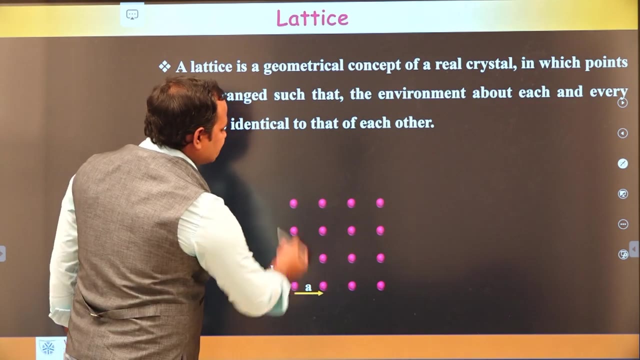 So a lattice means so. a lattice is a geometrical concept of real crystal in which the points are arranged such that the environment about each and every point is same. So that means what is the meaning is So, for example, this is the lattice that we constructed for some real crystal. 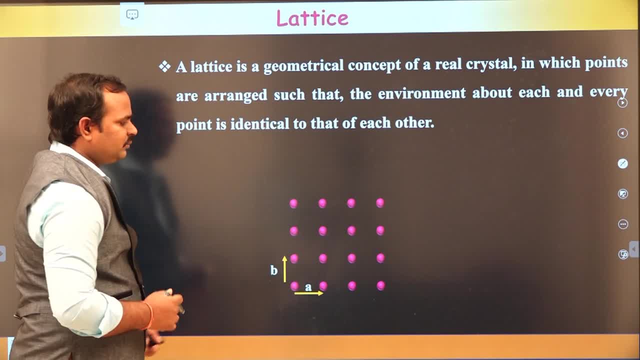 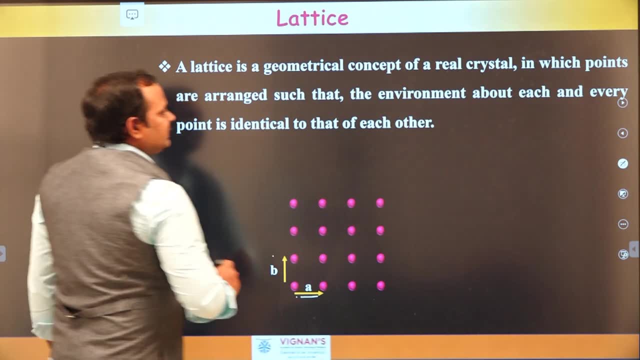 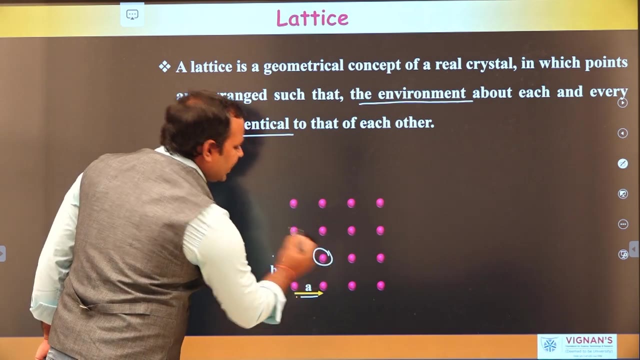 This is the lattice we constructed for some real crystal. Here the translational vectors are A and B And here the condition is the environment about. each and every point is identical. That means, for example: let us consider: this is the point I am taking. 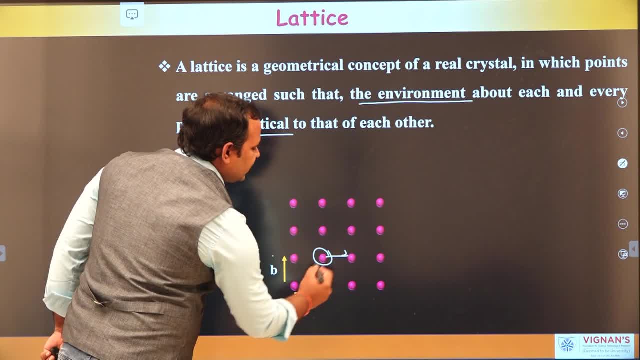 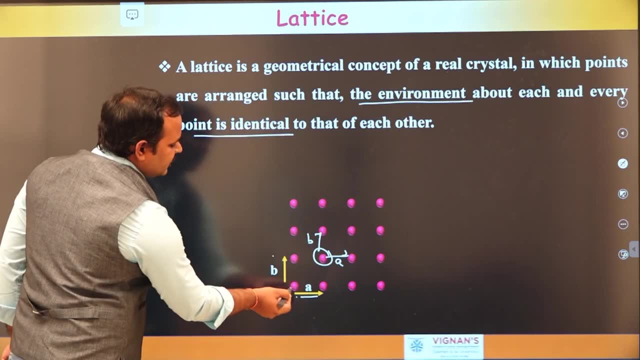 And let us see: the distance between the two successive points in this direction is A And the distance between the two successive points in this direction is B, Which is similar. For example, if you take this is the same At the A distance. we have another point. 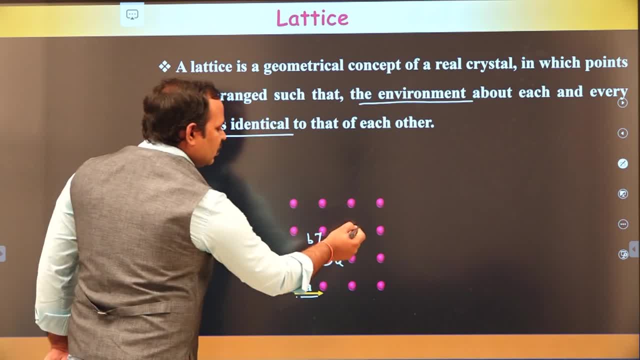 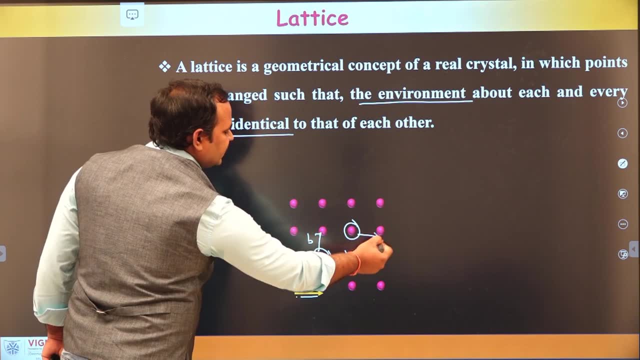 At the B distance. we have another point in this direction. Similarly, we can also take any atom. The distance between the two successive atoms in the X direction is A, And the distance between the two successive atoms in the Y direction is B. 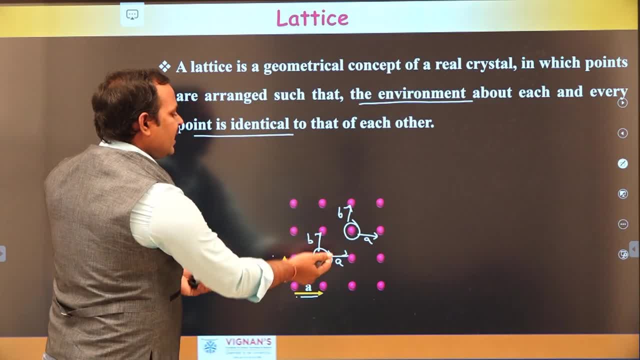 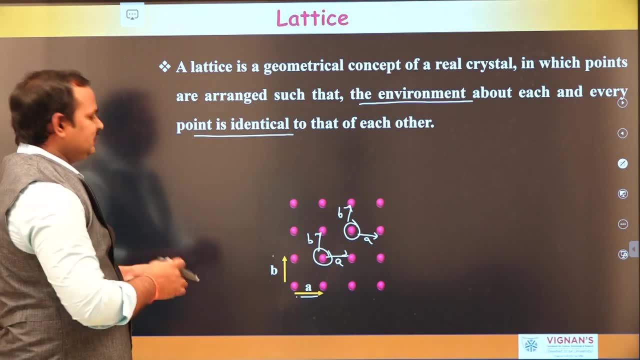 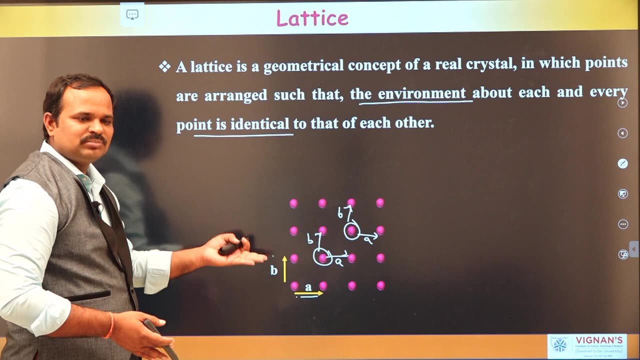 That means the environment about each and every atom is identical to each other. So this is called a lattice, This lattice. this is only a point. Now, these points, if you replace with the atoms in the crystal, we get a total crystal structure. 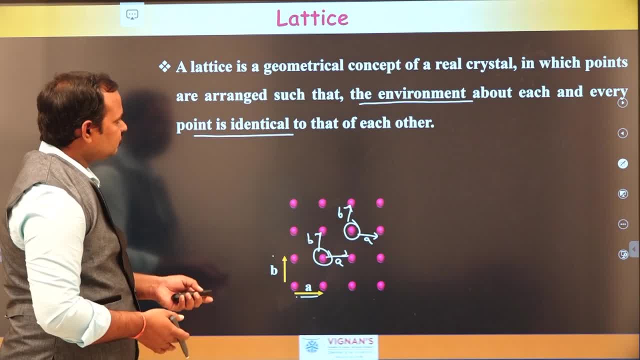 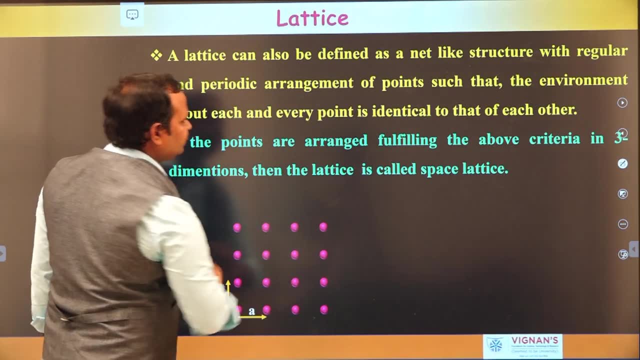 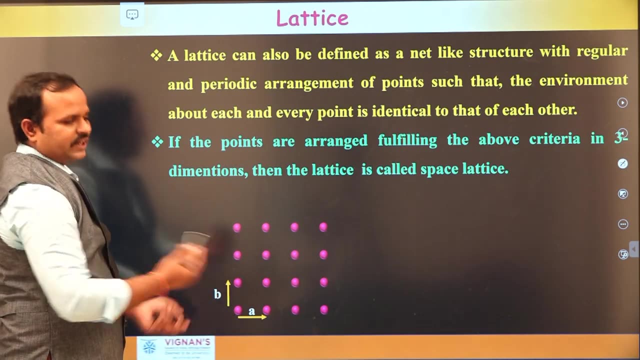 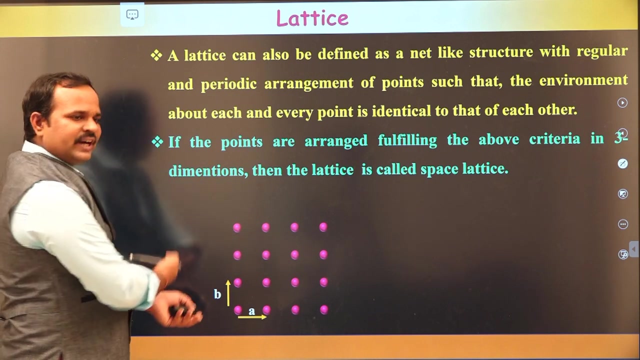 You will get more clear as you go on. So a lattice can also be said as a net-like structure with regular, periodic arrangement of points in space, such that the environment about each and every point is identical, For example, if you replace these atoms, if you continue, I mean if you fulfill these atoms in three dimensions. 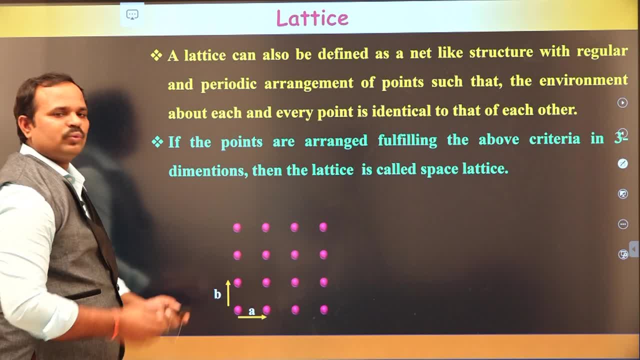 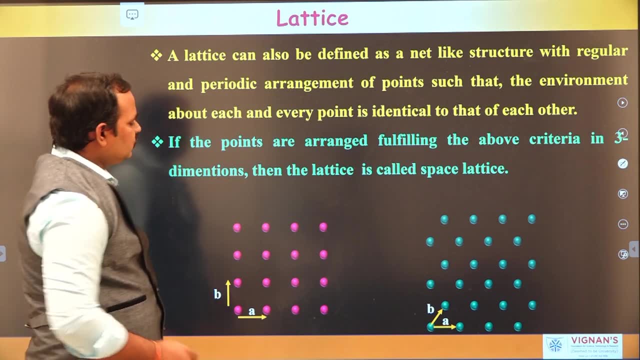 we get a space lattice. This is a two-dimensional lattice. We also get a three-dimensional lattice that is called a space lattice. So, as I told you, the lattice no need to be only having these two. We also have translational vectors in another direction. 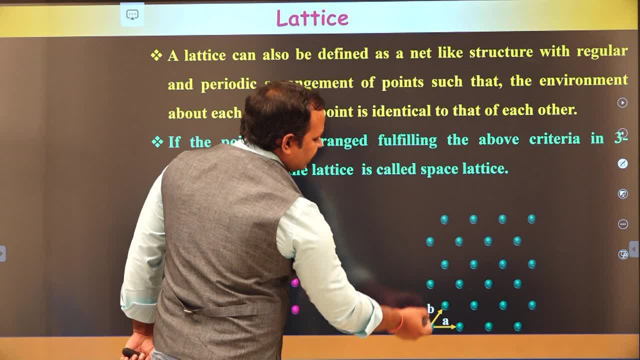 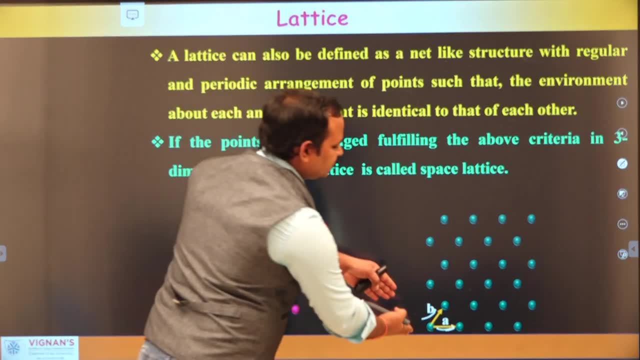 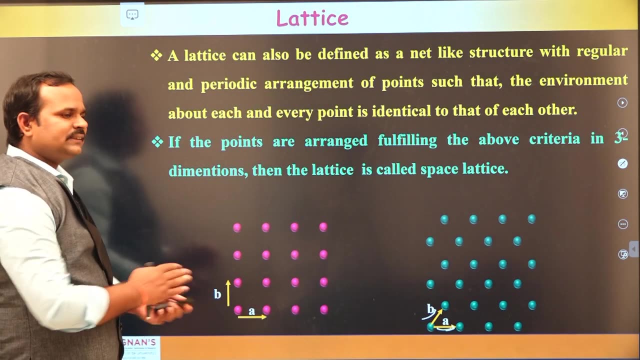 In this case, this is another space lattice where the translational vectors are taken in this direction and in this direction Now repeat these atoms with the translational vectors in these directions to get a total crystal structure. So this is the lattice. 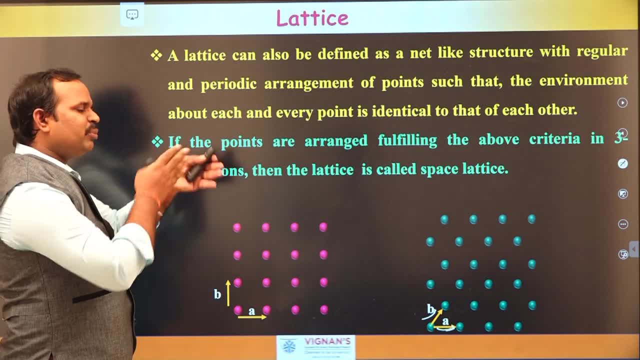 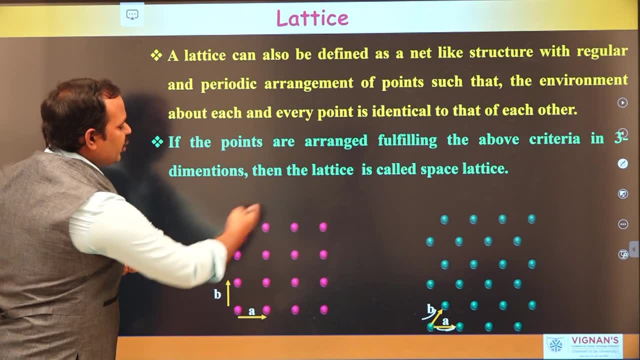 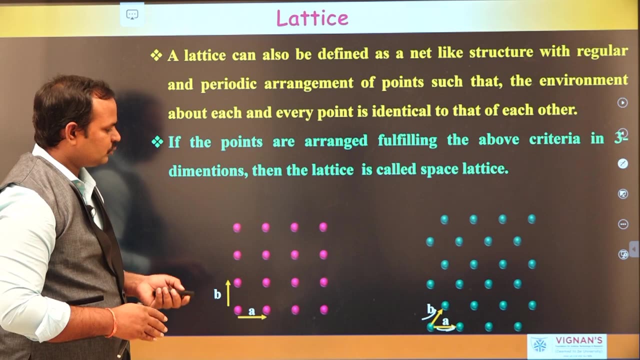 Lattice gives you just points in the space. They are only points which correspond to a real crystal. Now, each and every point, if you replace with the corresponding crystal atoms, we get a total crystal structure. Let's see what is that. 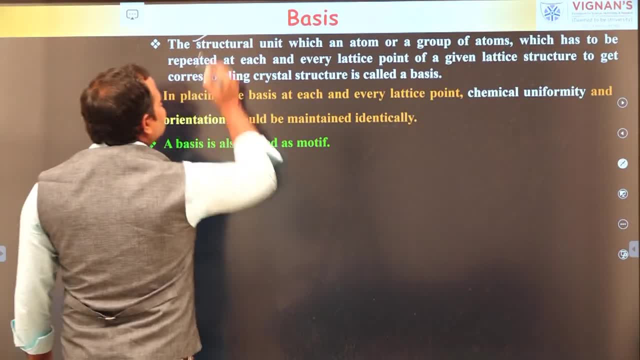 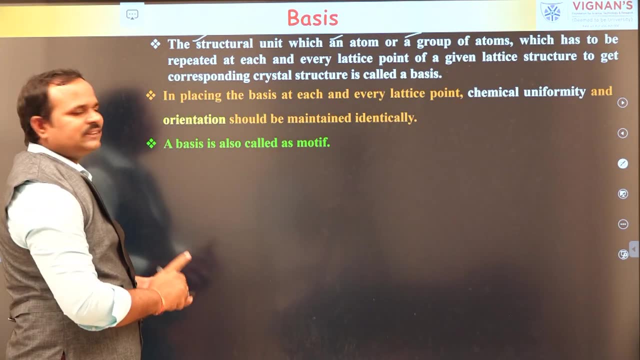 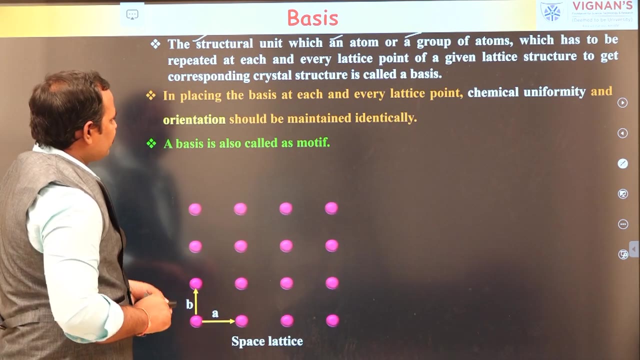 That is called a basis. So a basis is a structural unit with an atom or a group of atoms which has to be repeated at each and every lattice point to get a total crystal structure, For example. let us see what is actually the meaning of this basis. 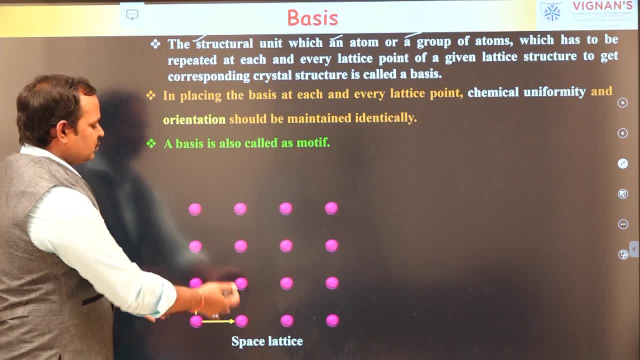 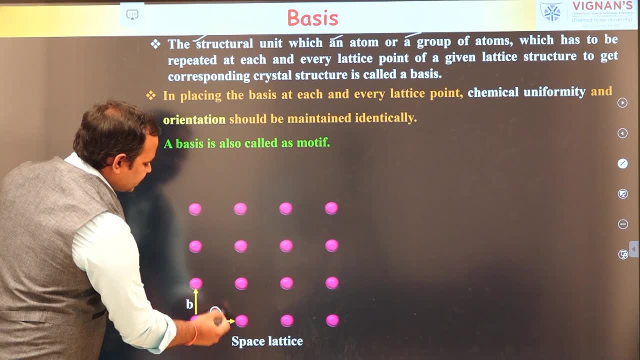 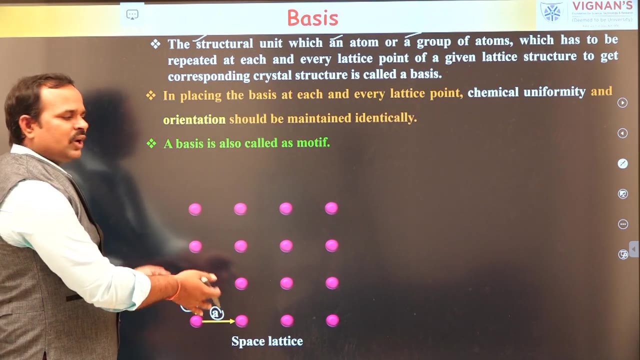 This is a space lattice for some crystal which was generated by using a translational vector and operator, with a translational vector a in x direction, with a translational vector b in y direction. Now these are only points in the space. Now to get a total crystal structure we need some basis. 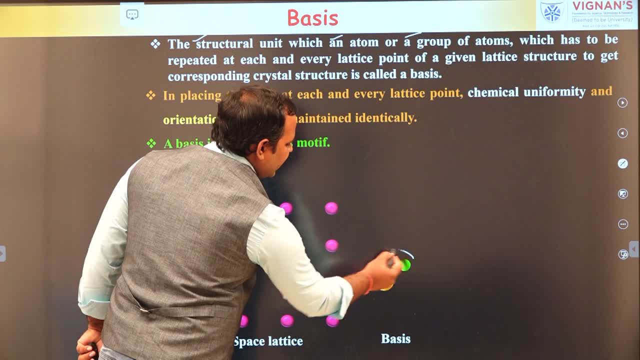 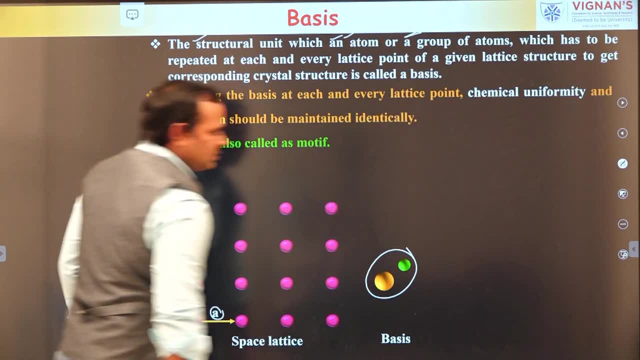 The basis here is: this is the basis. There are two atoms are there. That means this is a structural unit with one atom or a group of atoms. It can be one atom or two atoms or a group of atoms. This is a structural unit. 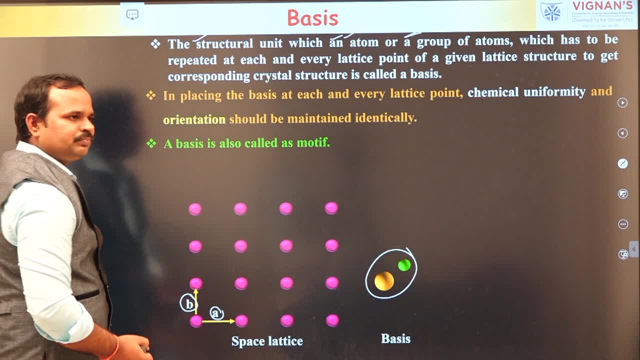 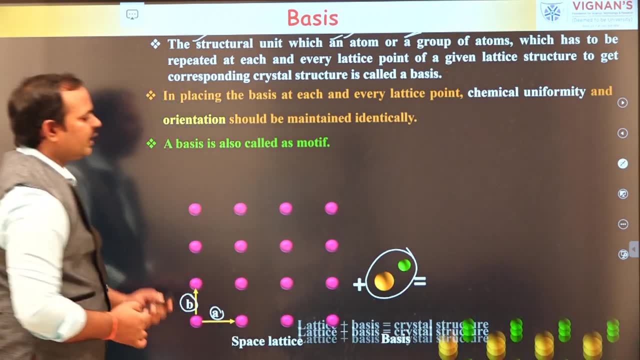 Now what we do is we take these atoms and replace with the lattice points. So now we replace these atoms at each and every lattice point to get a total crystal structure like this way. So that means, if you see, this is the structural unit. 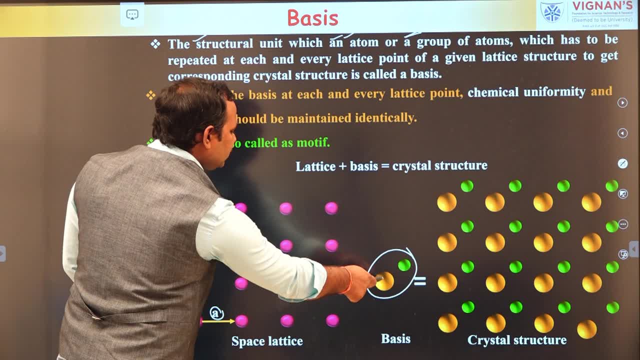 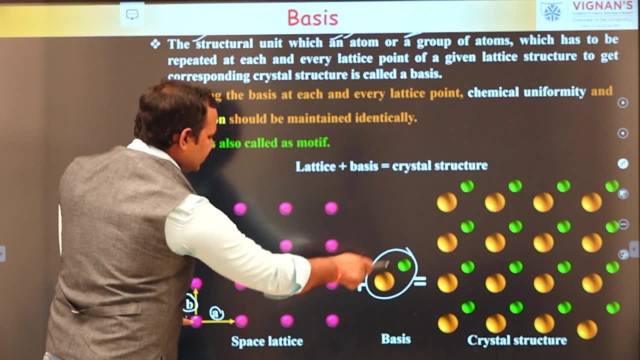 That means these are the atoms in my crystal structure. Now these crystal structure atoms are placing at each and every lattice point. This is the point. So we are replacing this point with these two. So we get these two Now for this point again replaced. 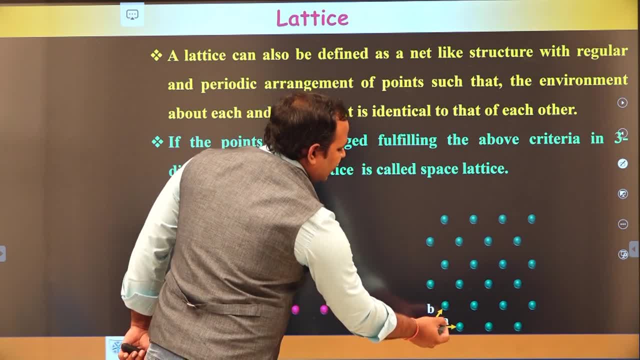 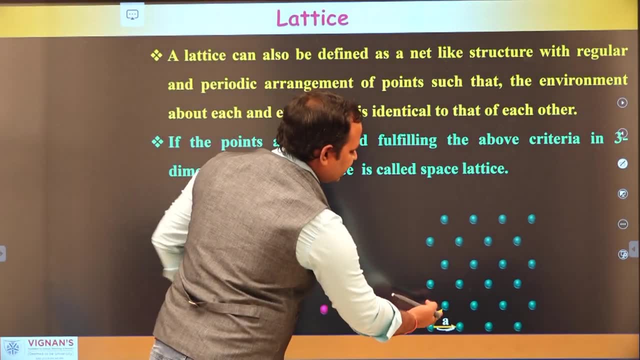 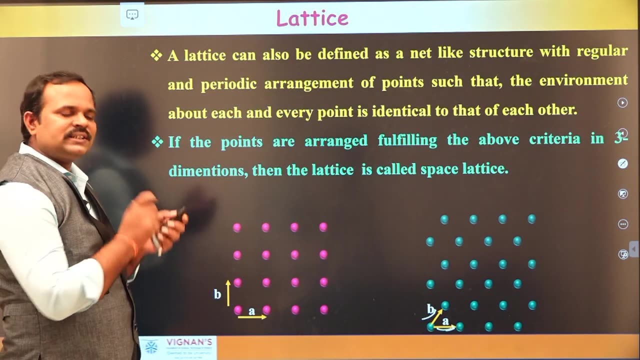 this is another space lattice where the translation vectors are taken in this direction and in this direction. Now repeat these atoms with the translational vectors in these directions to get a total crystal structure. So this is the lattice. Lattice gives you just the. 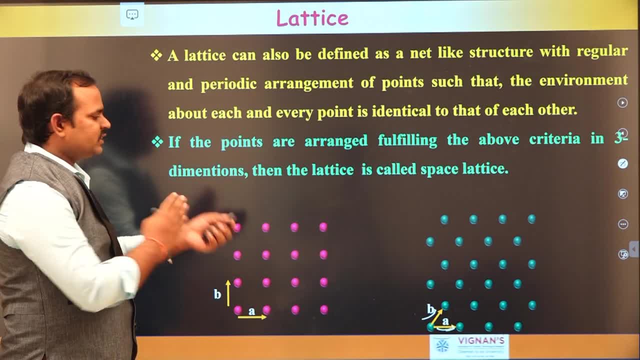 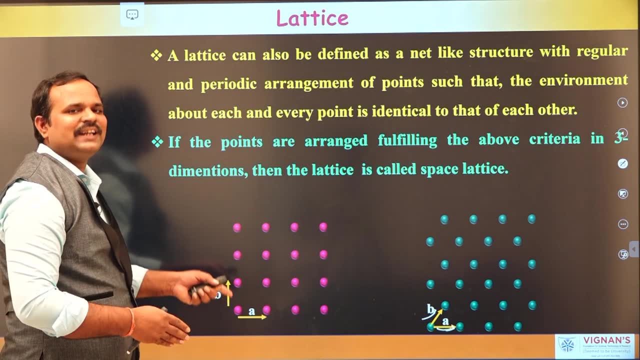 points in the space. They are only points which correspond to a real crystal. Now, each and every point, if you replace with the corresponding crystal or round atoms, we get a total crystal structure. Let's see what is that. That is called a. 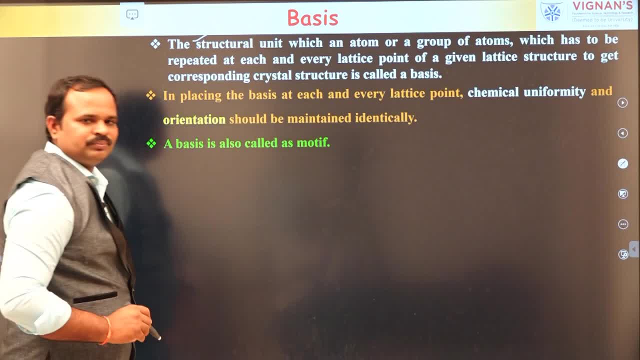 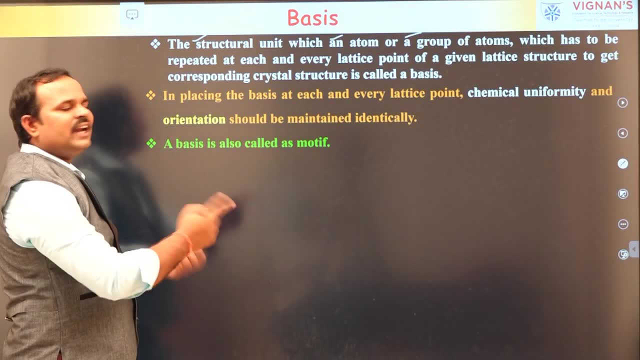 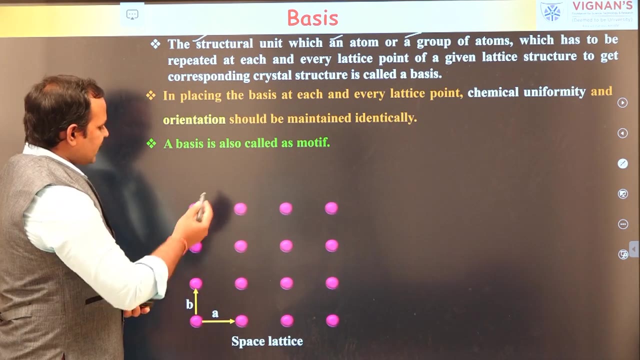 basis. So a basis is a structural unit with an atom or a group of atoms which has to be repeated at each and every lattice point to get a total crystal structure, For example. let us see what is actually the meaning of these spaces. This is the space lattice for some crystal which was generated by 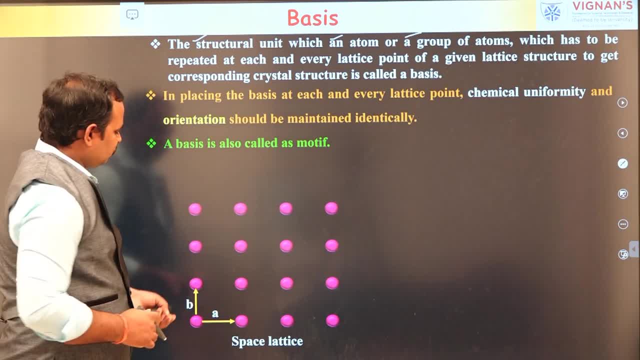 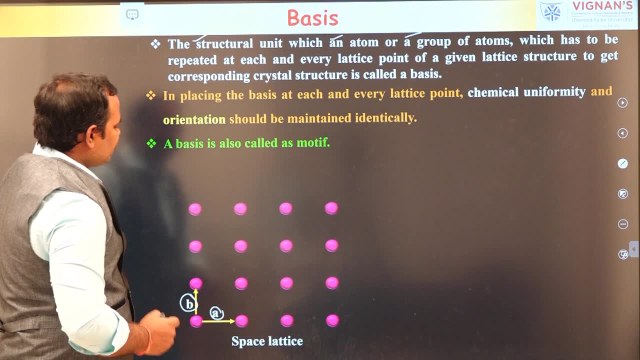 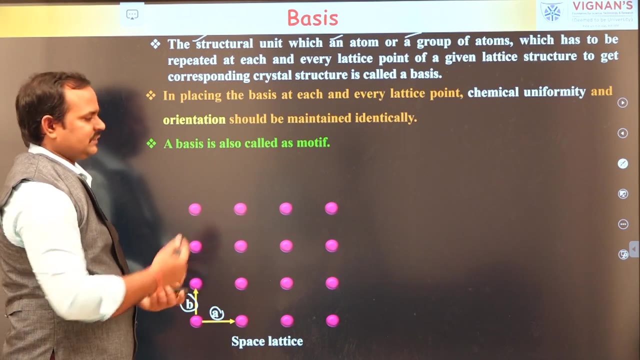 using a translational vector and operator, With a translational vector A in X direction, with a translational vector B in the Y direction. Now, these are only points in the space. Now, to get a total crystal structure, we need some basis. The basis here is: this is the basis: There are two atoms. are there That? 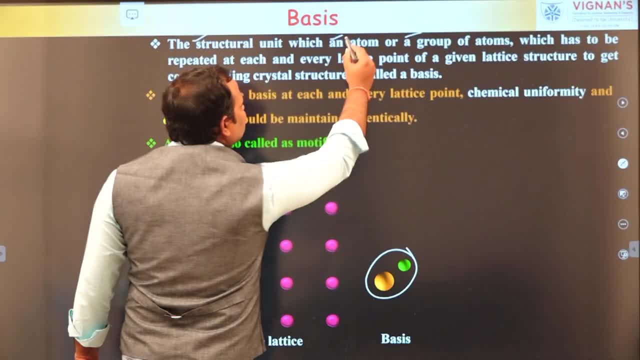 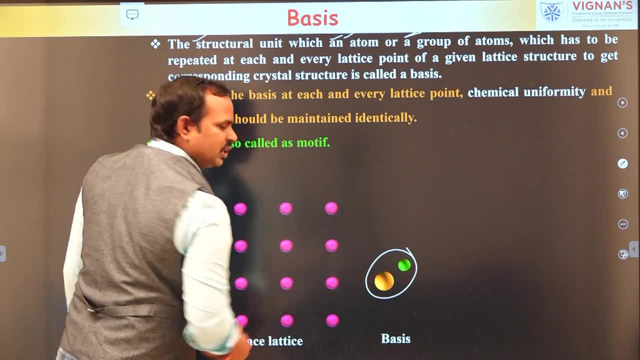 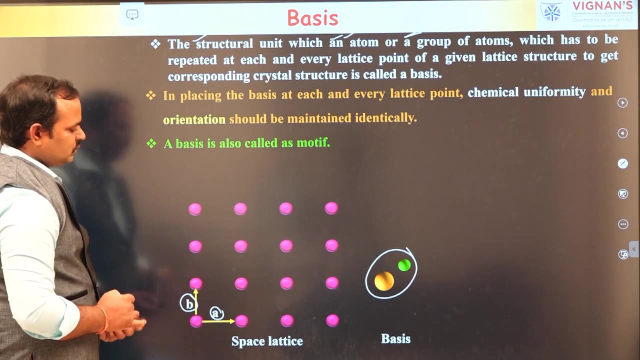 means this is a structural unit With one atom or a group of atoms. It can be one atom or two atoms or a group of atoms. This is a structural unit. Now what we do is we take these atoms and replace with the lattice points. So now we replace these atoms at each and every. 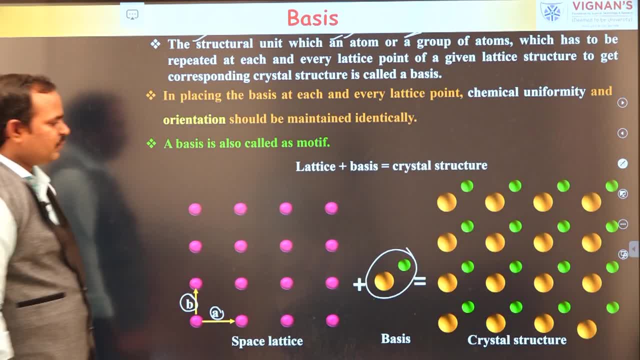 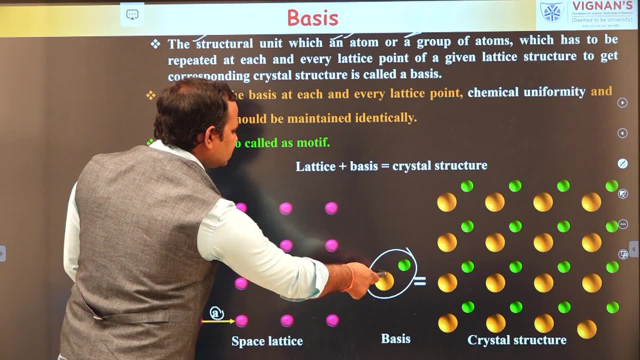 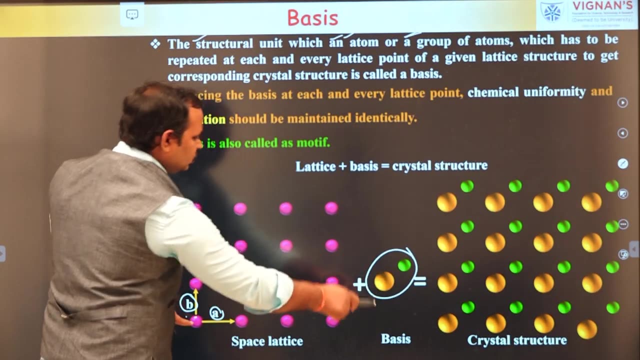 lattice point to get a total crystal structure like this way. So that means, if you see, this is the structural unit. That means these are the atoms in my crystal structure. Now these crystal structure atoms are placing at each and every lattice point. This is a point, So we are replacing this point with these two. 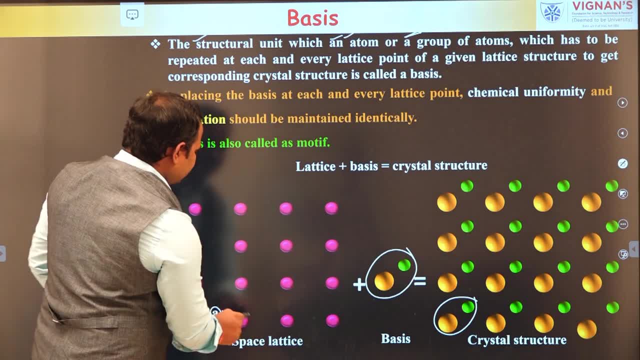 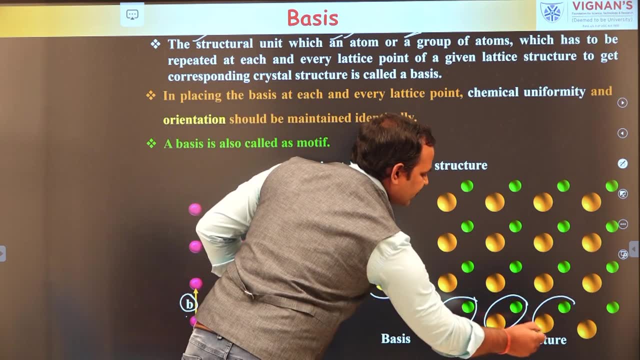 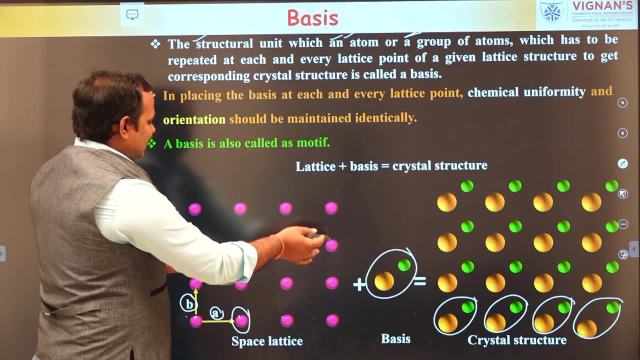 So we get these two Now for this point again replaced. So we get these two, And for this point we have these atoms, And for this point we have these atoms. So that means, at each and every lattice point, if we replace with the base atoms, we get a total crystal structure. 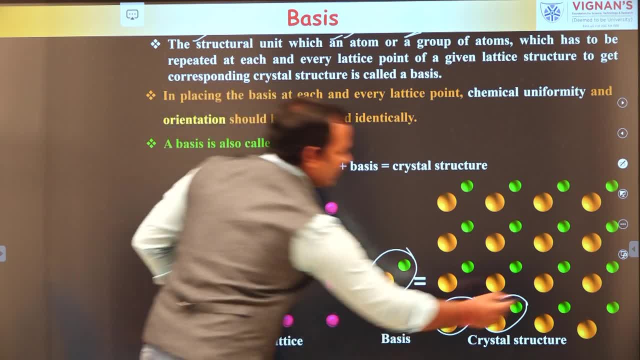 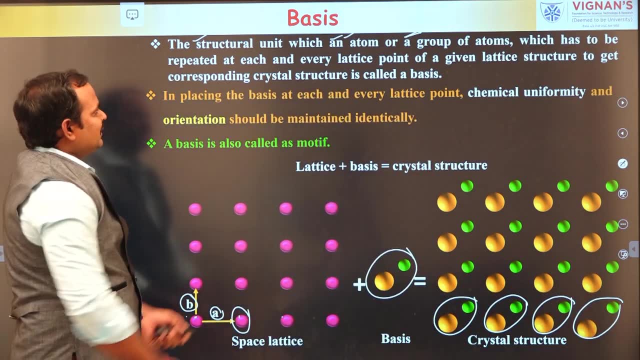 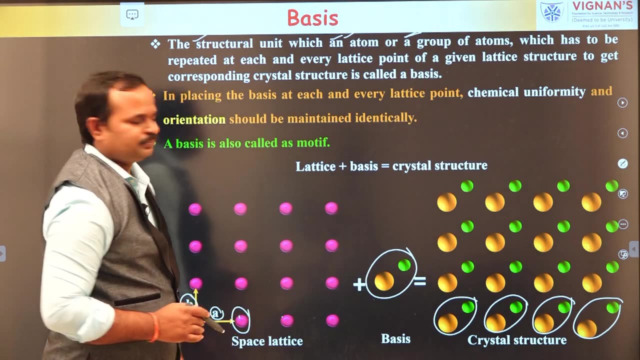 So we get these two, And for this point we have these atoms, And for this point we have these atoms. So that means at each and every lattice point, if we replace with the base atoms, we get a total crystal structure. 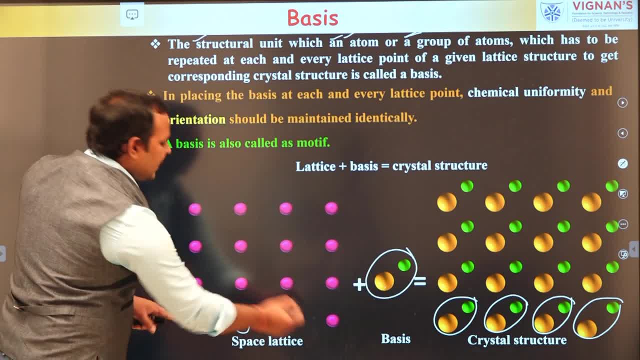 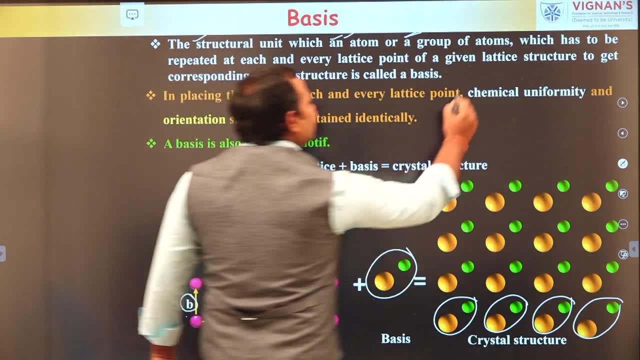 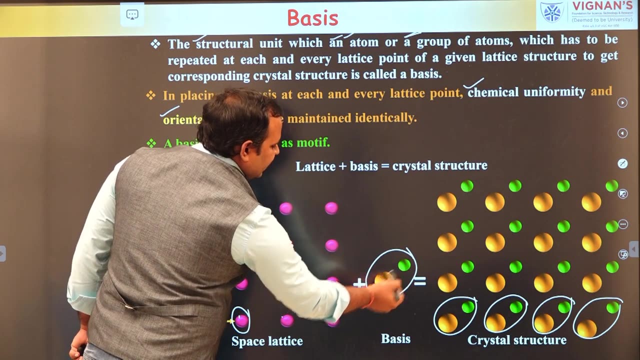 Here, in placing the bases at each and every lattice point, there are two important things needs to be understand. One is the chemical uniformity. Another one is orientation of the bases. If you see, the chemical uniformity means this is the two different atoms. 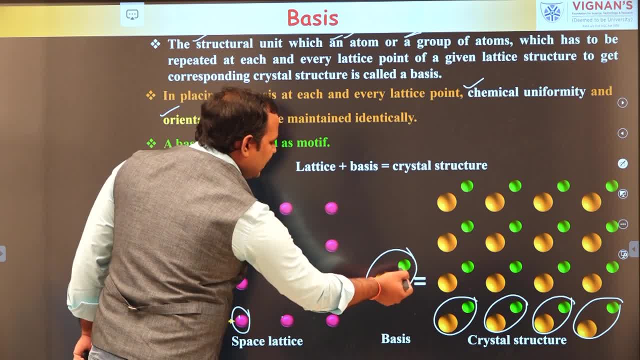 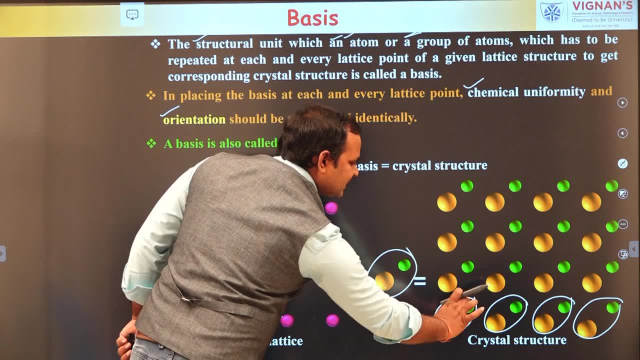 That means this crystal is a diatomic crystal. Now, while placing these two atoms at each and every lattice point- the chemical uniformity that means how they are there- they should be the same way. we should keep at each and every lattice point. 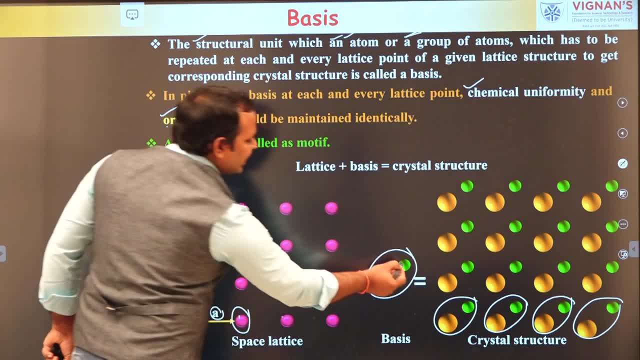 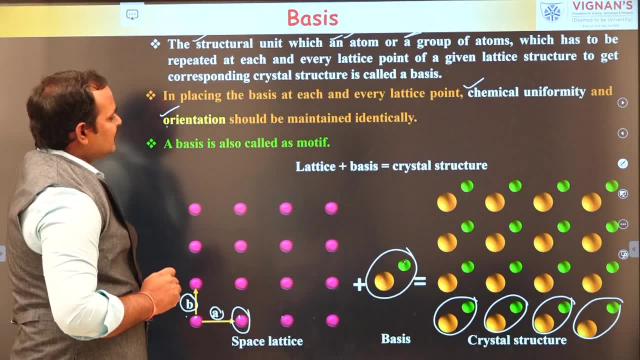 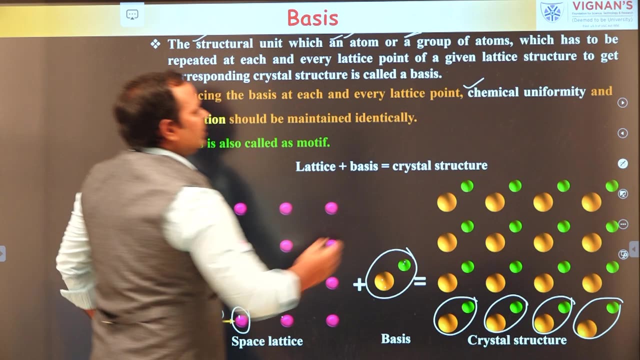 And also the orientation. For example, if you replace this atom with this one and with this one, then we won't get a total crystal structure. So that means when we place the bases atom at the lattice points we must keep chemical uniformity of the bases. 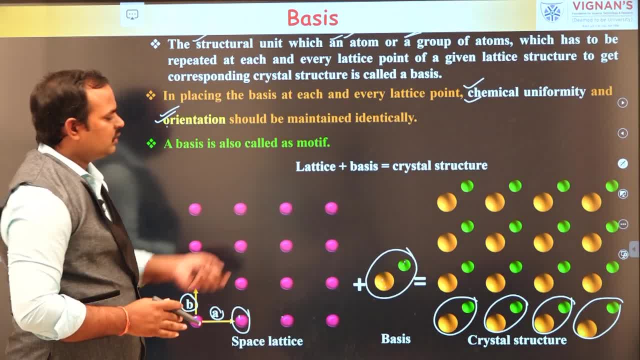 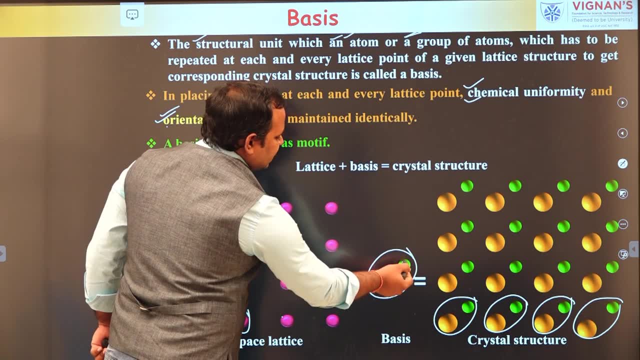 and the orientation of the bases is very important to get a total crystal structure. For example, if you replace, if you have a chemical non-uniformity, that means if you replace this atom with this one, then we may have a disordered crystal. 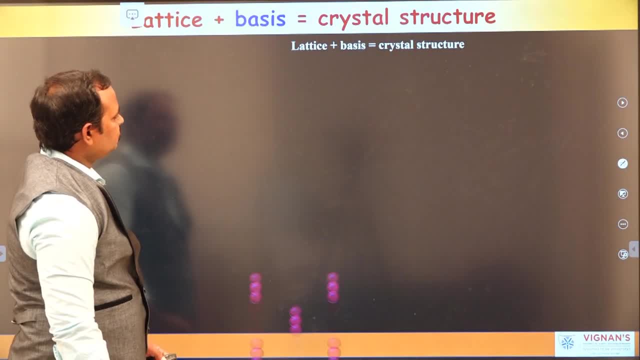 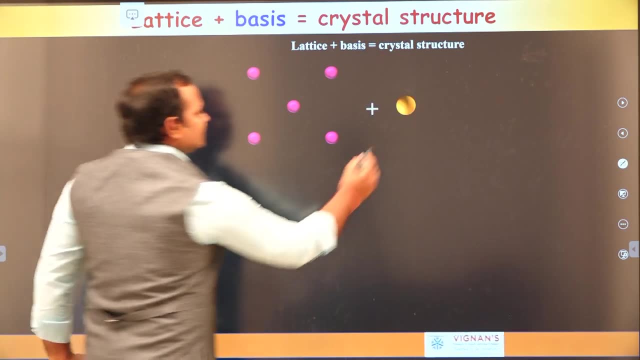 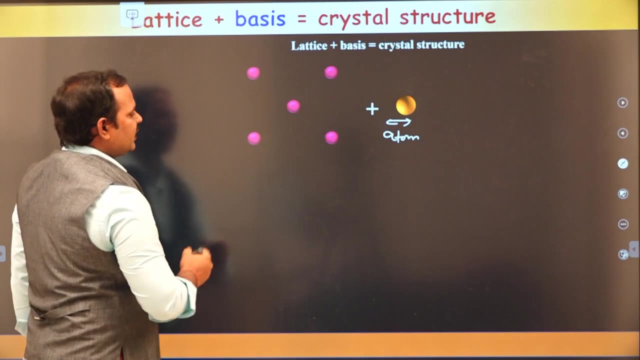 Let's see some more examples. So this is the lattice that I have constructed for some crystal, And this is the bases. Now this is the atom in the crystal. This is a monatomic crystal. That's why we have only one atom. 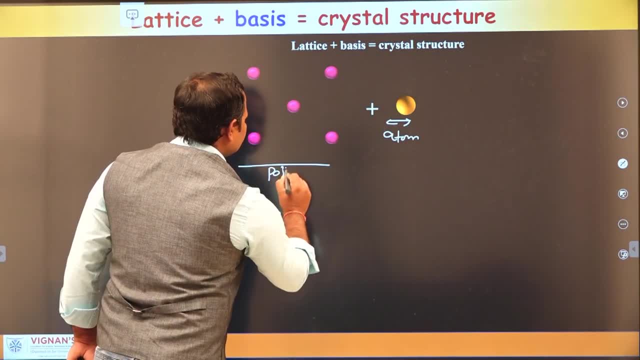 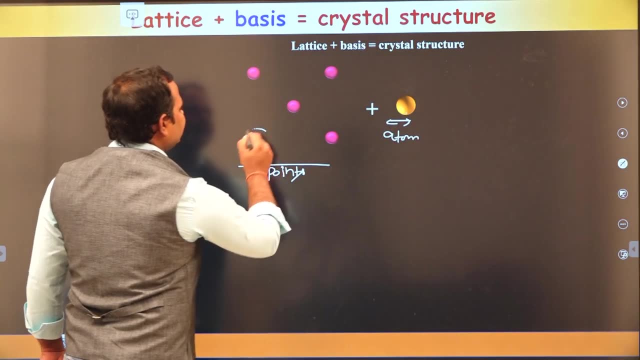 This is the lattice, This is the points. These are only points in space. Now, at each and every lattice point, we replace this point with the atom, So we get a crystal structure, For example. if you see, this is an atom. 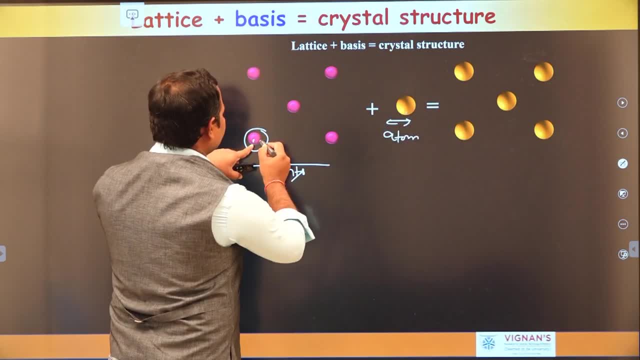 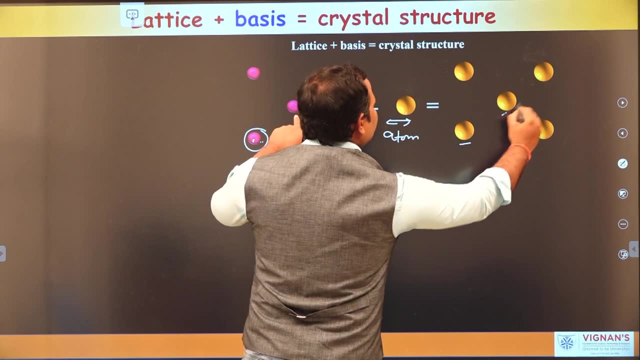 This is a point, This is an atom. So replace this point with this atom. with this point, We get this atom. At this point, we have another atom. At this point, we have another atom. At this point, we have another atom. 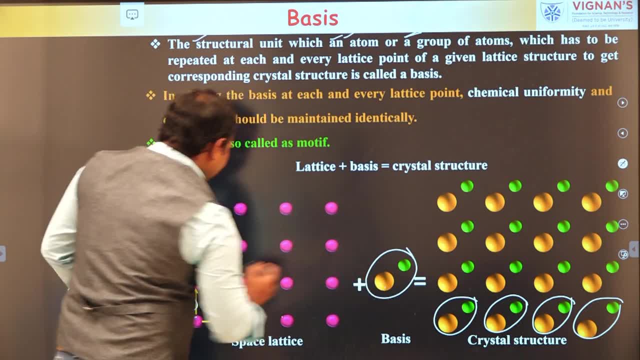 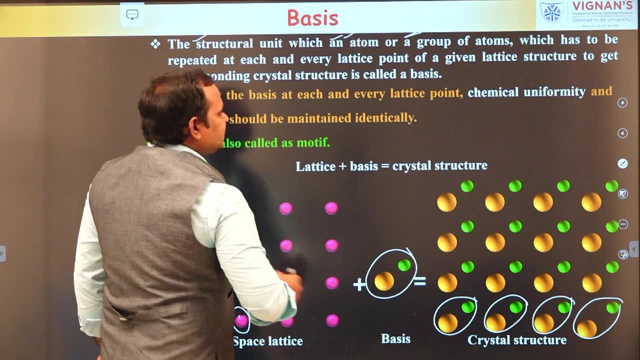 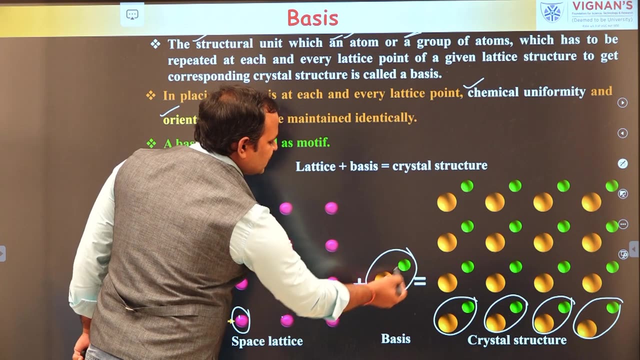 Here, in placing the bases at each and every lattice point, there are two important things needs to be understood. One is the chemical uniformity. Another one is orientation of the bases. If you see, the chemical uniformity means this is the two different atoms, That means this crystal. 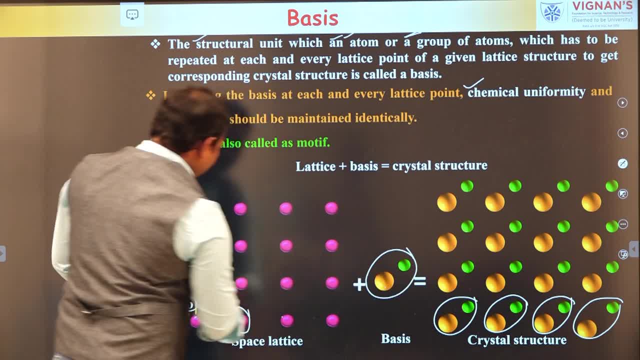 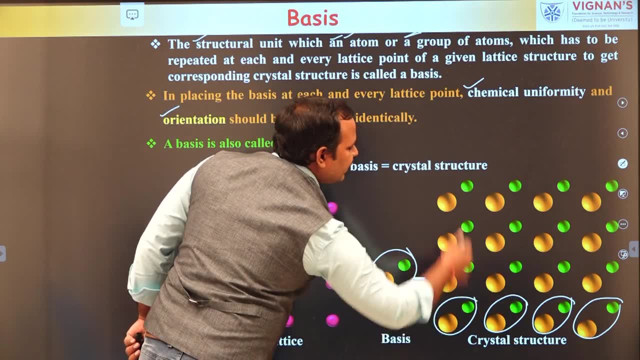 is a diatomic crystal. Now, while placing these two atoms at each and every lattice point, the chemical uniformity that means how they are there. So this is the same way we should keep at each and every lattice point, And also the orientation, For example, if you replace this atom with this one and with this one. 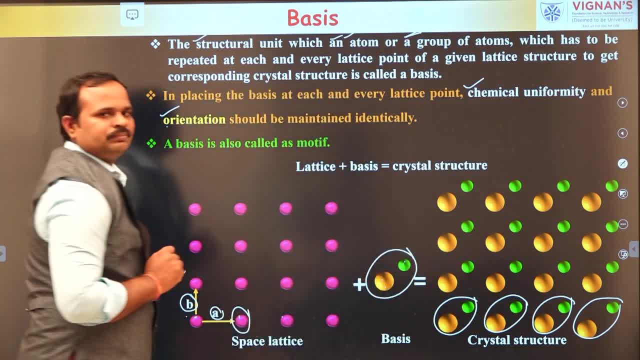 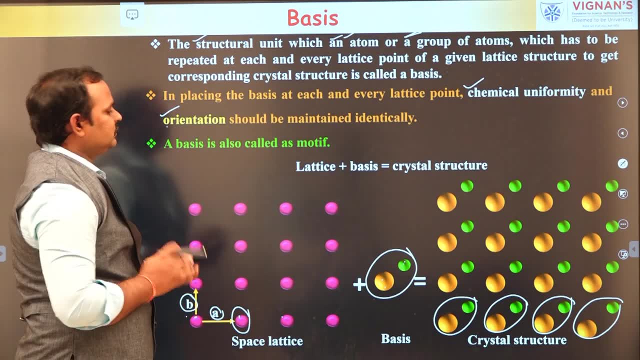 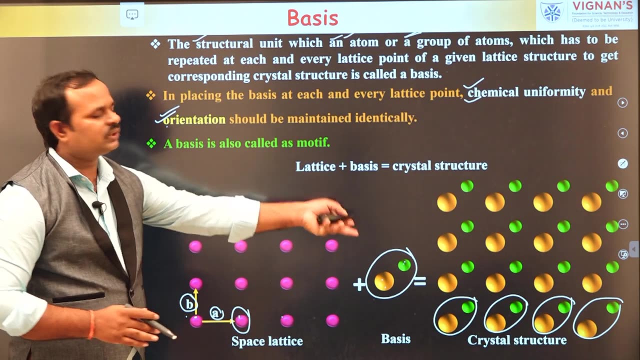 then we won't get a total crystal structure. So that means when we place the bases atom at the lattice points we must keep chemical uniformity of the bases, and the orientation of the bases is very important to get a total crystal structure. For example, if you have a chemical non uniformity, that means 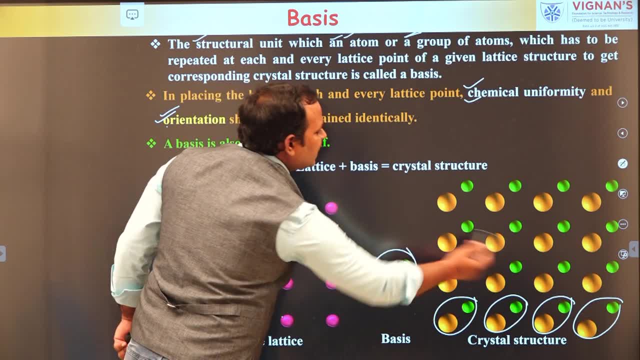 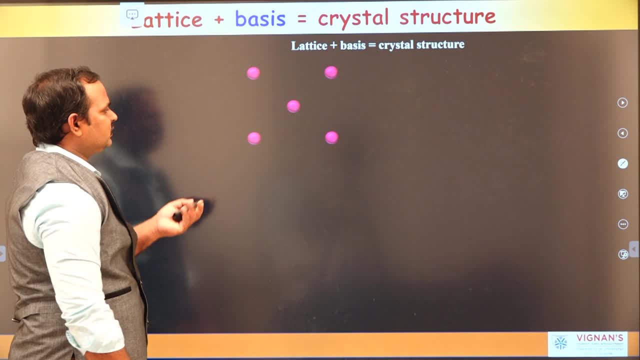 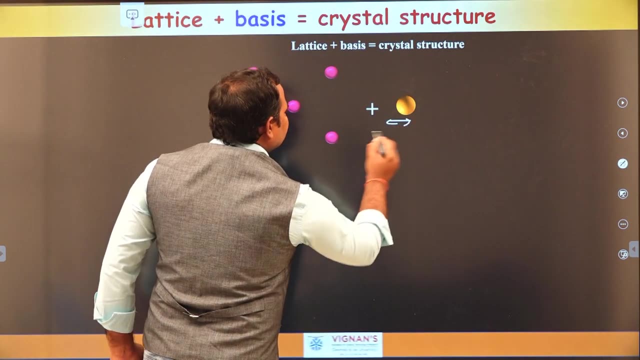 replace this atom with this one, then we may have a deserted crystal. Let's see some more examples. So this is the lattice that I have constructed for some crystal, and this is the basis. Now this is the atom in the crystal. This is a. 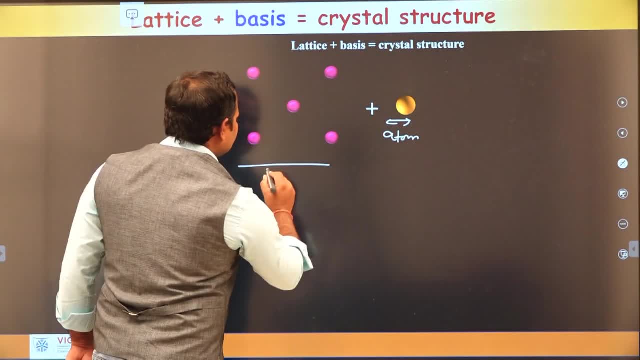 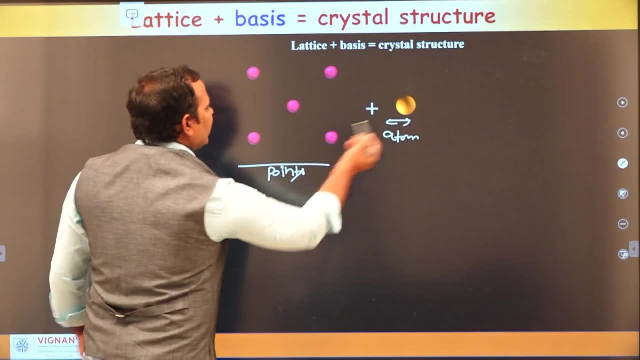 monatomic crystal. that's why we have only one atom. This is the lattice. This is a point. These are only points in space. Now, at each and every lattice point, we replace this point with the atom, So we get a crystal structure. 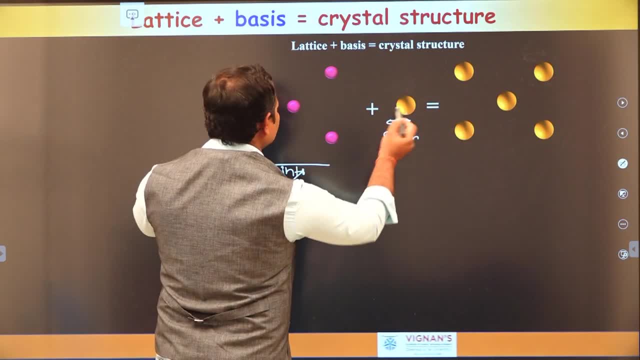 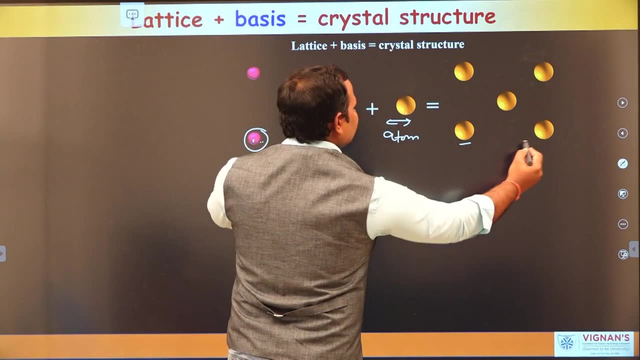 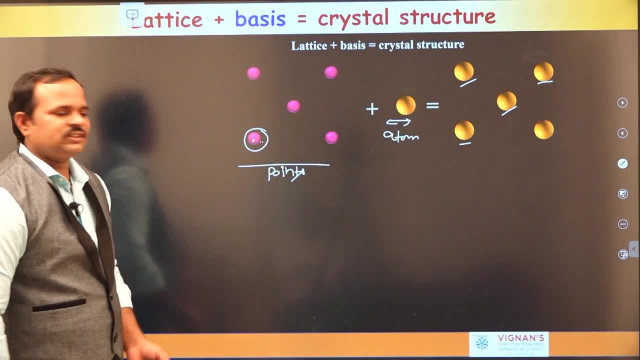 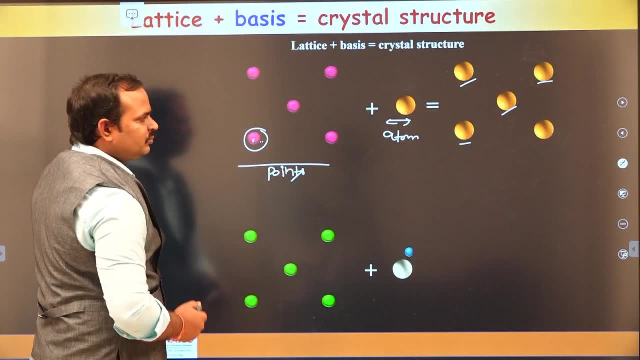 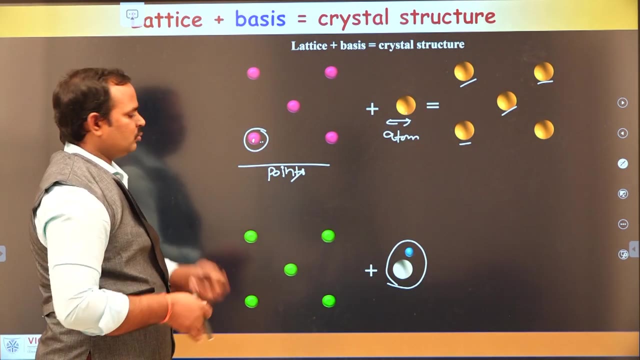 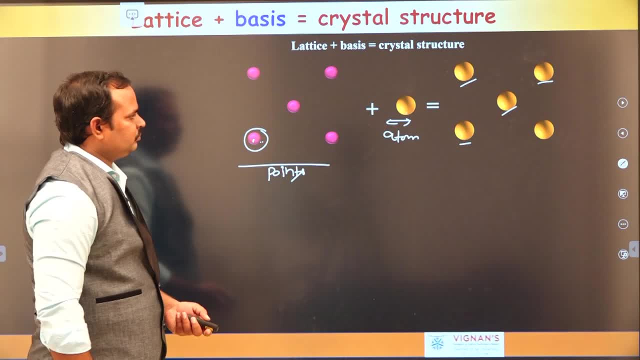 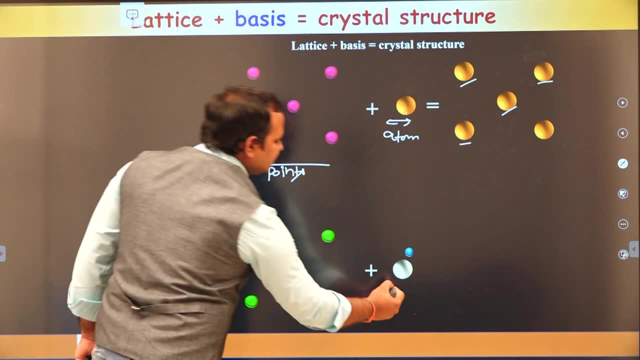 At this point we have another atom, So we get a crystal structure. Similarly we also have diatomic molecules, For example in the same lattice. if your basis is two atoms, it can be even more, two or group of atoms even more. 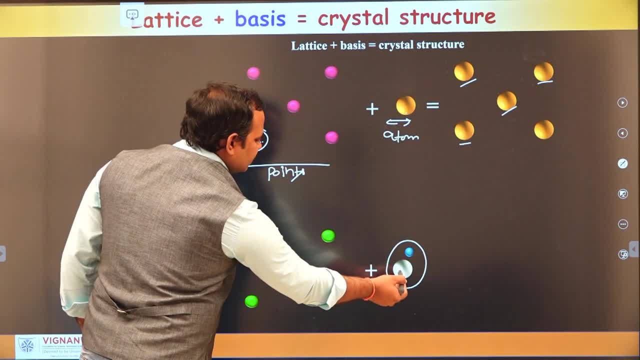 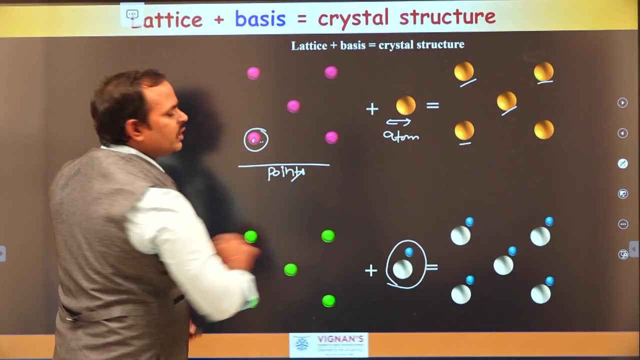 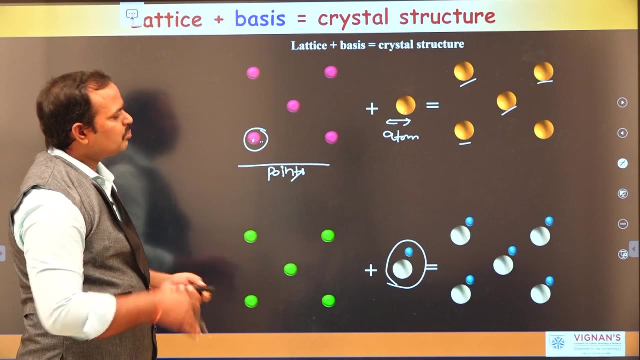 number of atoms. Now replace these base atoms at each and every lattice point to get a corresponding full crystal structure. This is how we get a corresponding crystal structure. That means lattice plus base gives you crystal structure. We will see some more examples. This is the lattice. 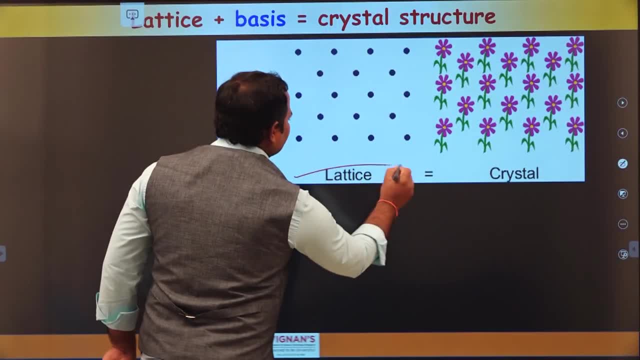 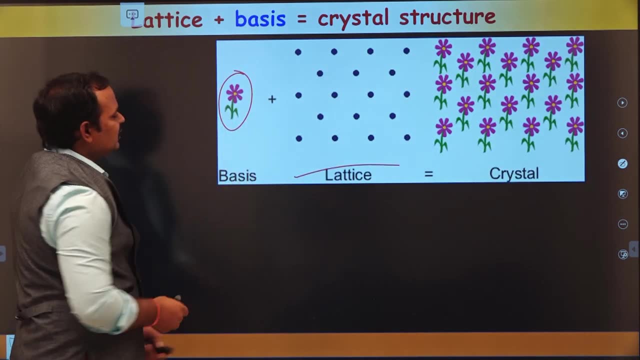 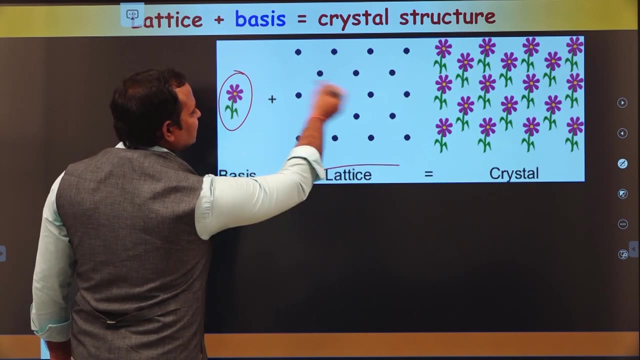 so this is the lattice that was constructed. Now, this is the basis. Of course, this is not an atom. this is only for the understanding purpose. Now, as per our theory, the basis should be replacing the lattice points and while replacing the chemical uniformity and orientation, should be: 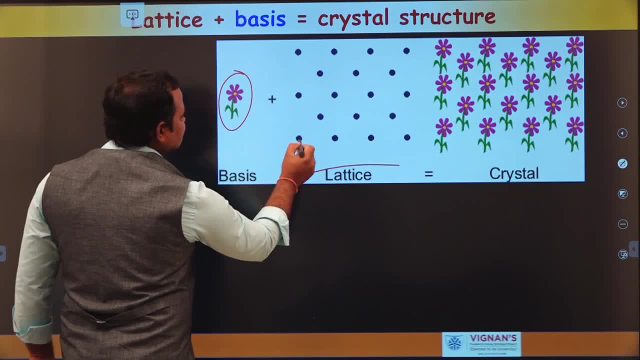 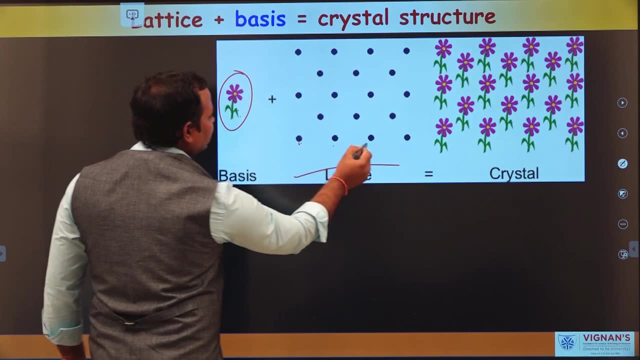 should be same or identical. Now replace this atom with this base at each and every point, So you keep this atom, this basis, at this point, this point, this point and this point, So we get total crystal structure. Now you can see when we are not changing their. 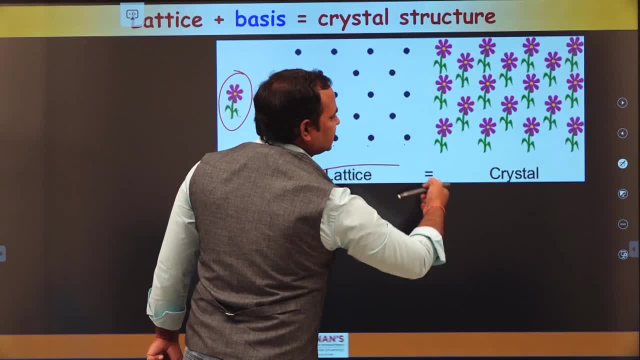 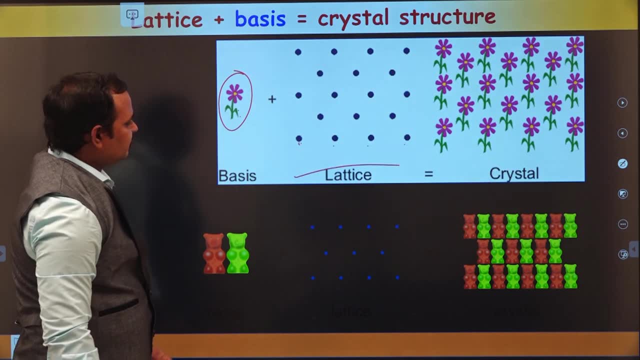 orientation and uniformity, we get total crystal structure as it is. For example, if you change, then you get a disorder crystal structure here. Similarly we also have another one. These are the points. If you see, this is a point, this is the. 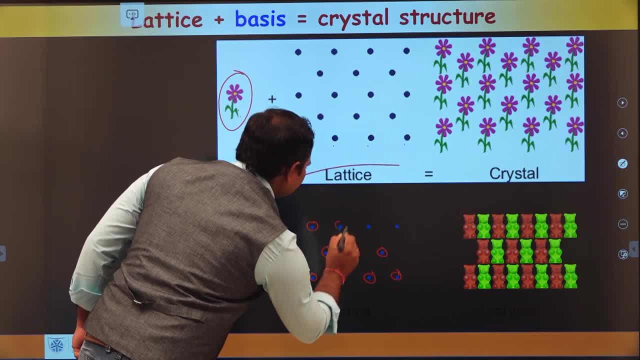 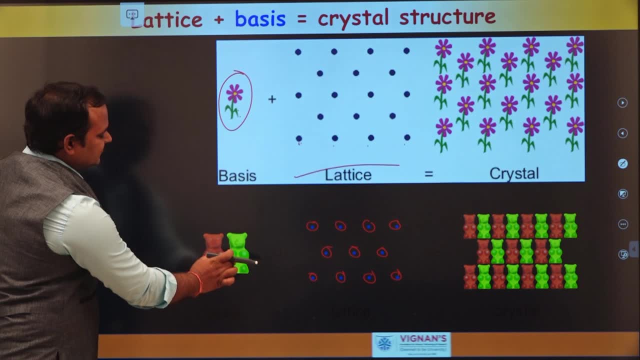 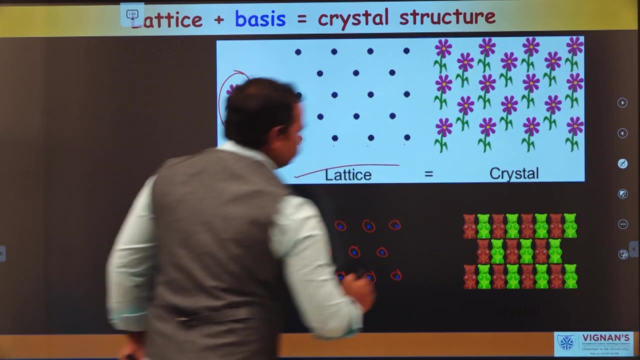 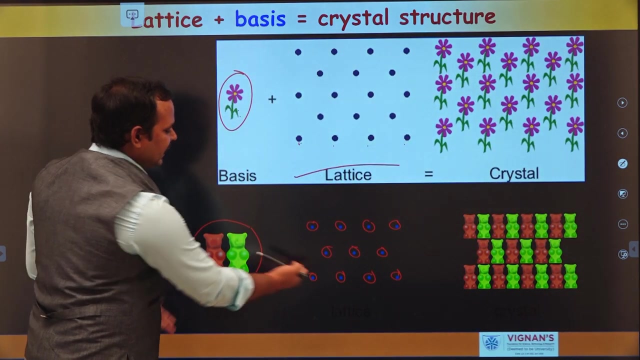 lattice points Now. this is the lattice point Now. these are the two dolls. One is red color and green color. Now replace these two dolls. This is the diatomic molecule. I can say there are two atoms are there Now, replace this basis at each and every lattice point. Now, when I'm 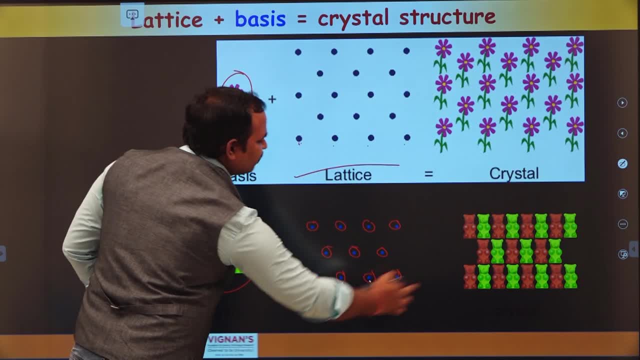 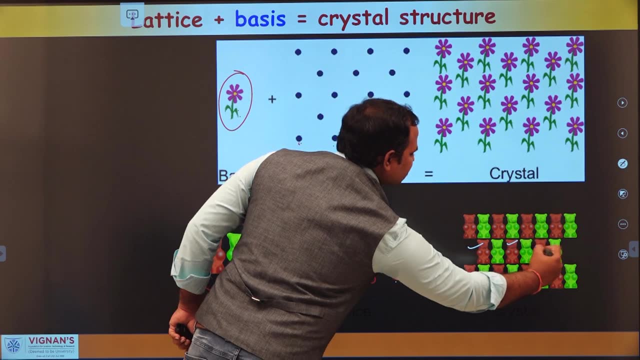 replacing this basis. at this point, this point, this point, we are getting total crystal structure. You can see there are only three points, So there are. this is the base atoms. this is the base atom. this is the base atom for the. 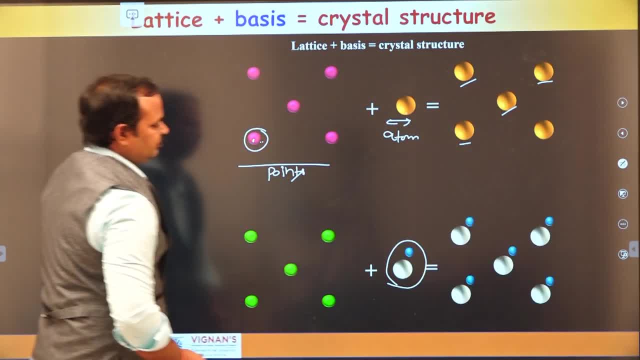 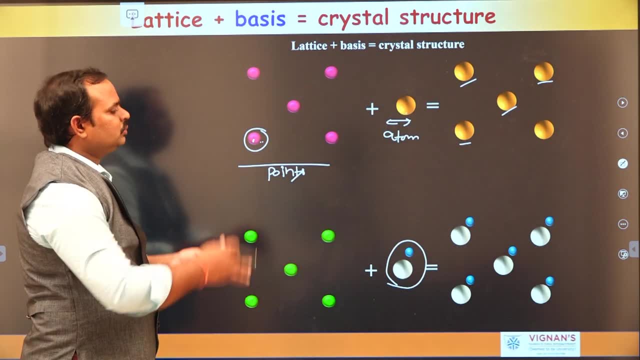 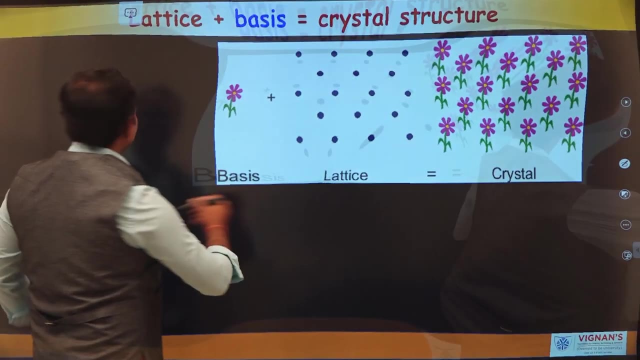 every lattice point to get a corresponding full crystal structure. This is how we get a corresponding crystal structure. That means lattice plus base gives you crystal structure. We will see some more examples. This is a. this is the lattice. So this is the. this is the. 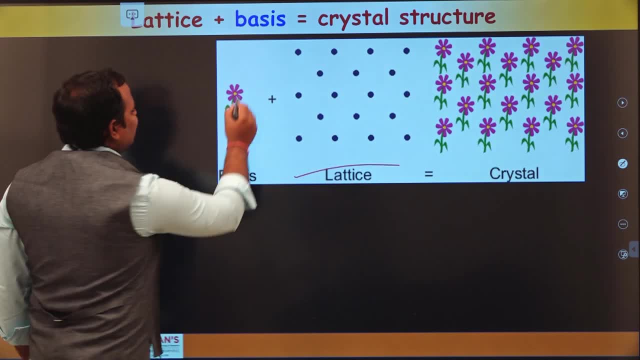 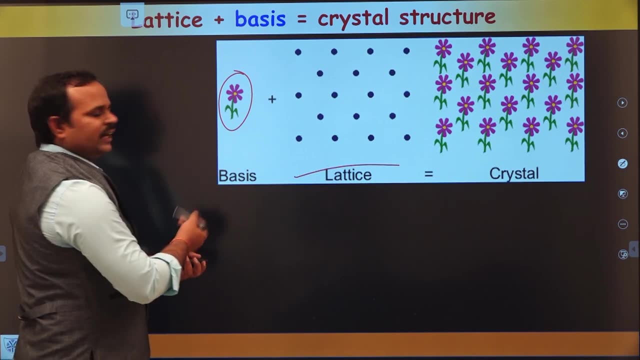 lattice that was constructed. Now, this is the basis. Of course, this is not an atom. This is only for the understanding purpose. Now, as per our theory, the basis should be replacing the lattice points and while replacing the chemical uniformity and orientation, should be: should be. 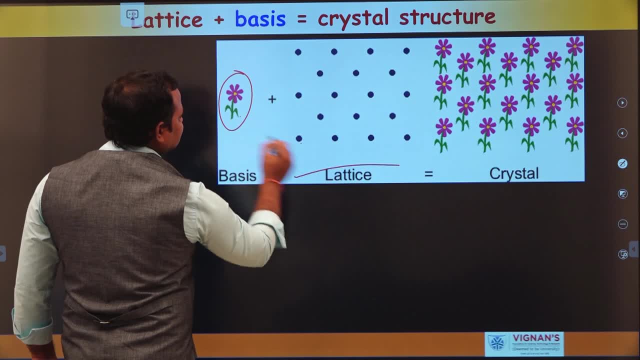 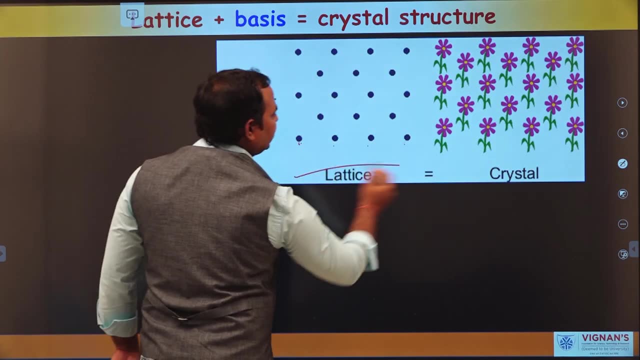 same are identical. Now replace this atom with this base at each and every point, So you keep this atom, this basis, at this point, this point, this point and this point. So we get total crystal structure. Now, as you can see when we are, 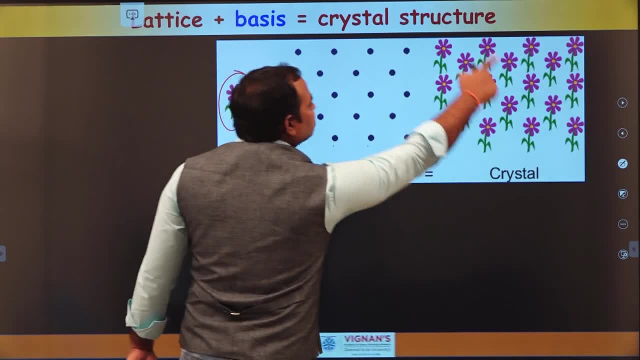 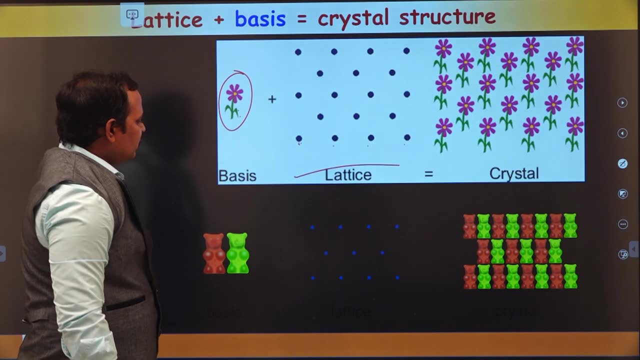 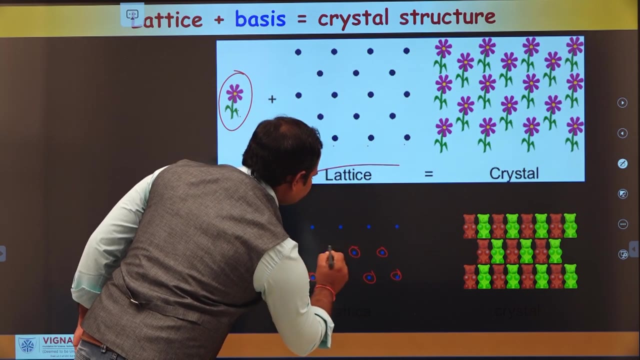 not changing their orientation and uniformity, we get total crystal structure as it is. For example, if you change, then you get a disorder crystal structure here. Similarly, we also have another one. These are the points. If you see, this is a point. This is the lattice points. Now, these are the two dolls. One is red color and green. 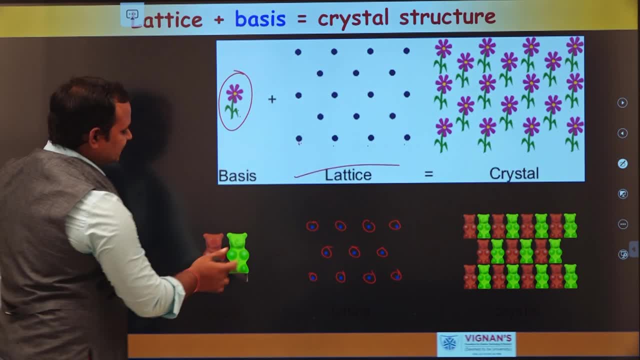 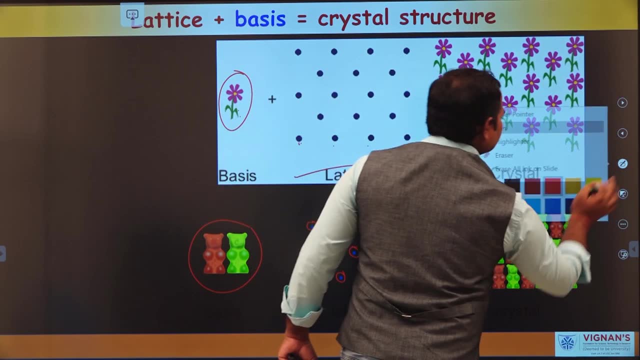 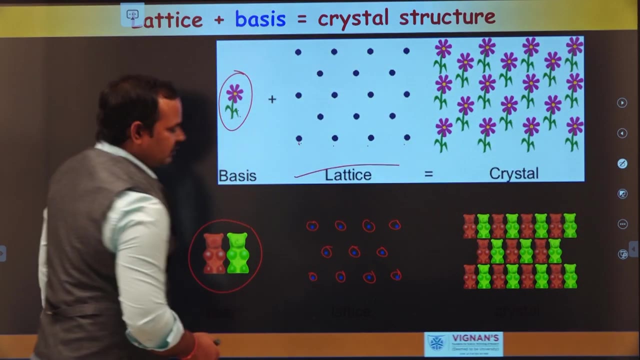 color. Now replace these two dolls. This is the diatomic molecule. I can say: there, two atoms are there Now. now replace this basis at each and every lattice point. Now, when I am replacing this basis at this point, this point, 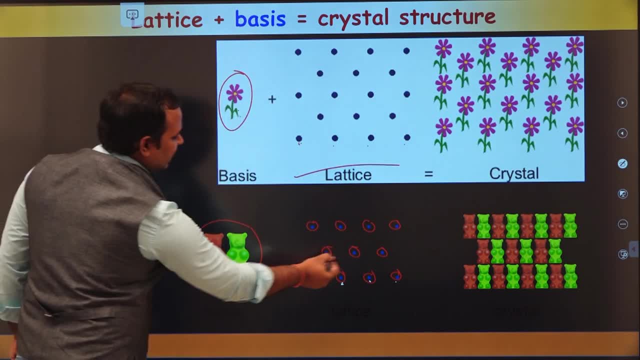 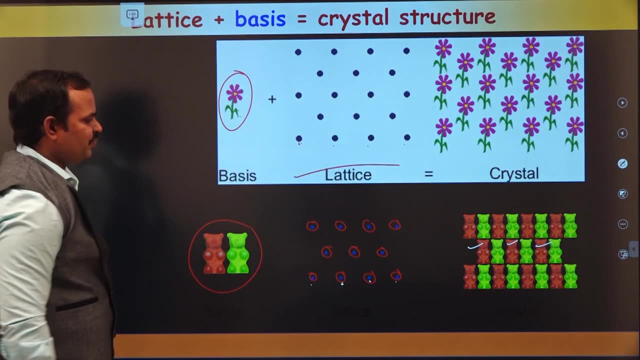 we are getting total crystal structure. You can see there are only three points. So there are. this is the base atoms. this is the base atom. this is the base atom for the central row Now in place. for example, if you replace with the red to: 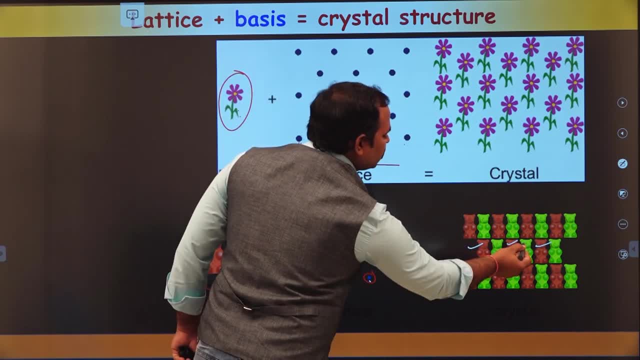 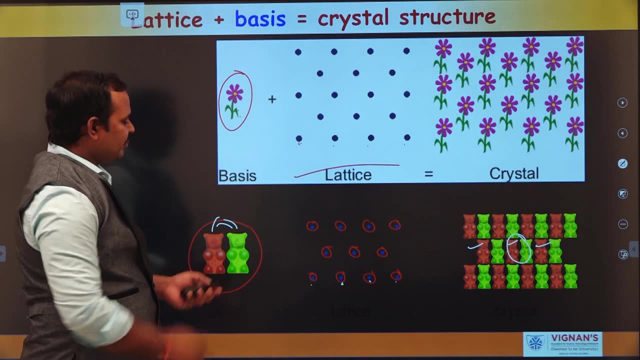 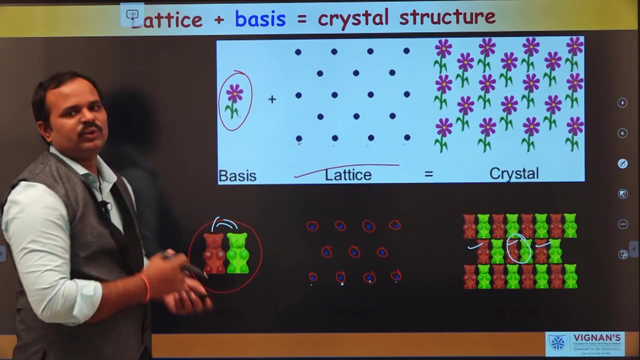 green, green to red, then at some point of time we may have interchanged atoms somewhere. that will give a disorder crystal. So that means when we are placing a basis at each and every lattice point we should mind the chemical uniformity and orientation. We will also see some more examples. This is: 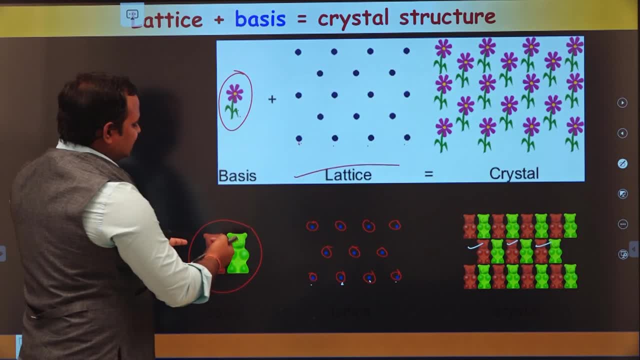 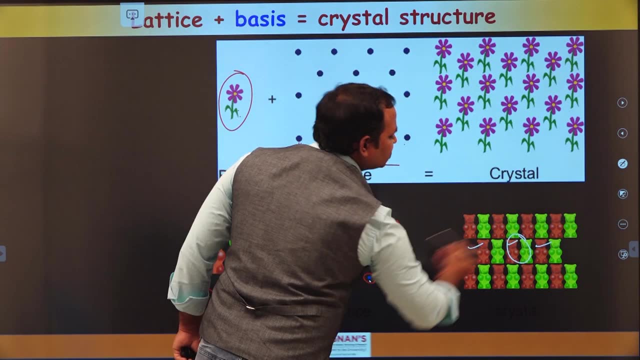 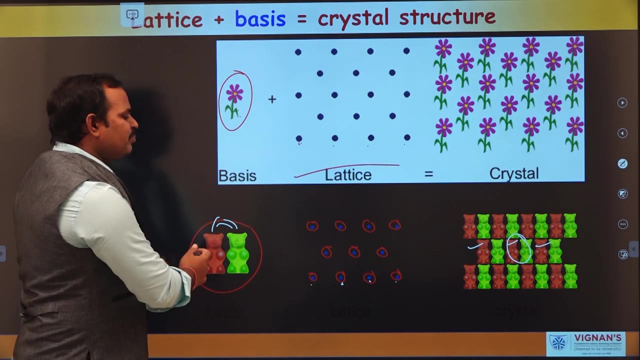 central row Now in place. for example, if you replace with the red to green, green to red, then at some point of time we may have interchanged atoms somewhere. That will give a disorder crystal. So that means when we are placing a basis at each. 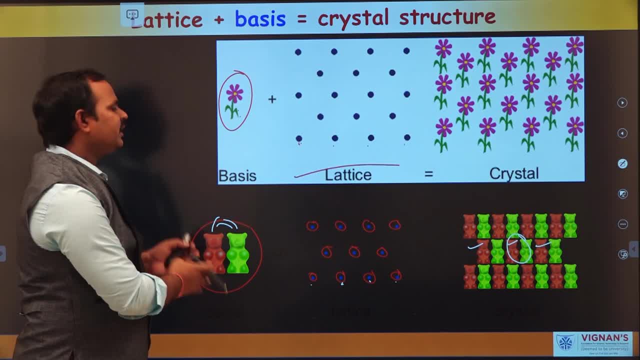 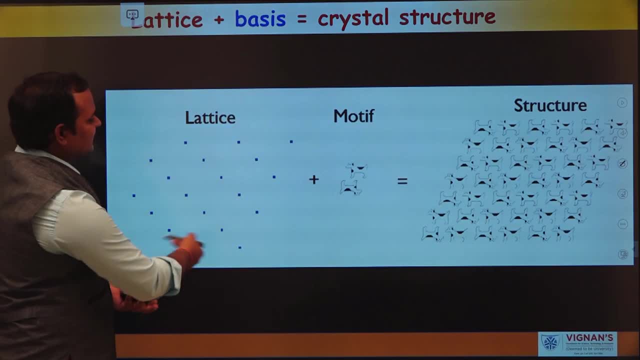 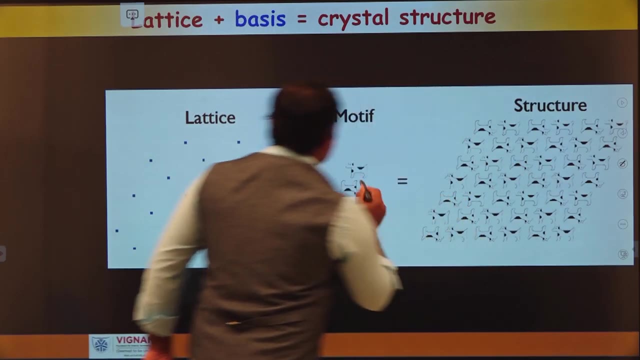 and every lattice point, we should mind the chemical uniformity and orientation. We'll also see some more examples. This is a lattice. This is a lattice constructed by using some translational vector. Here, this is a basis. Here, the basis is two dogs, small dogs which are 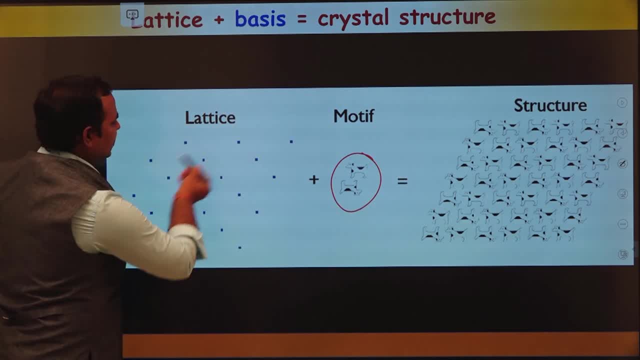 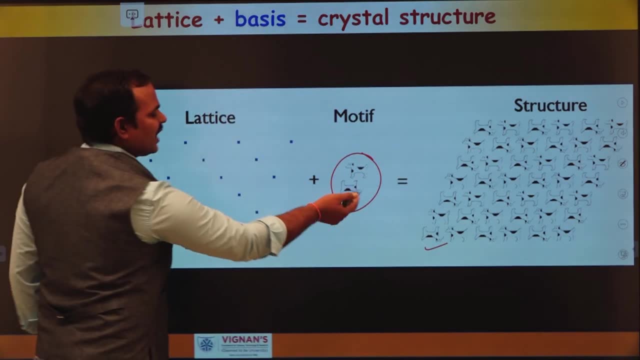 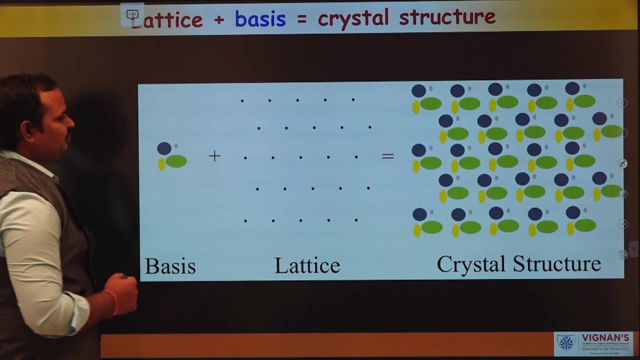 inverted. Now the basis. you need to keep at each and every lattice point to get total crystal structure. This is how you get a total crystal structure. In place of this, you can have two different atoms which are inverted. The another example is- this is one You can see here. this is the basis atoms. There are four atoms. 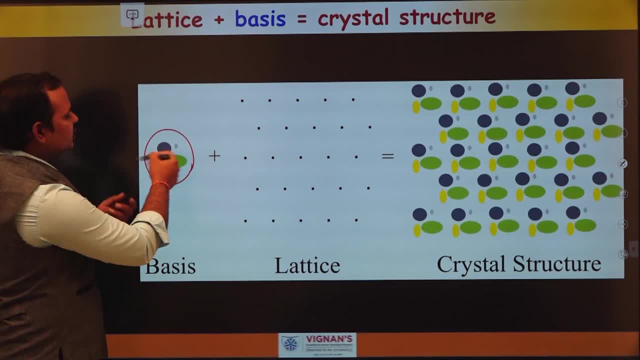 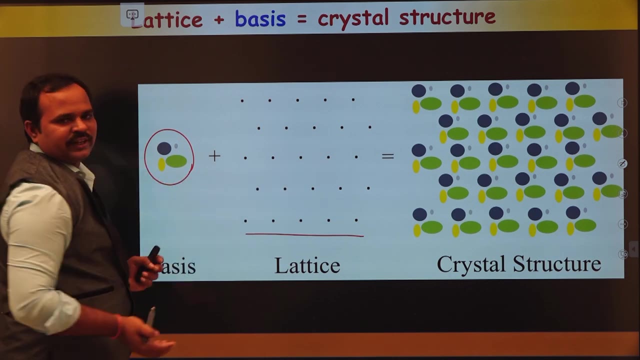 are there and also the dimensions of atoms are also different and also the distribution of atoms are also different. And this is the corresponding space lattice with different translational vectors in x and y directions. Now keep this basis at each and every lattice point. Now keep this at. 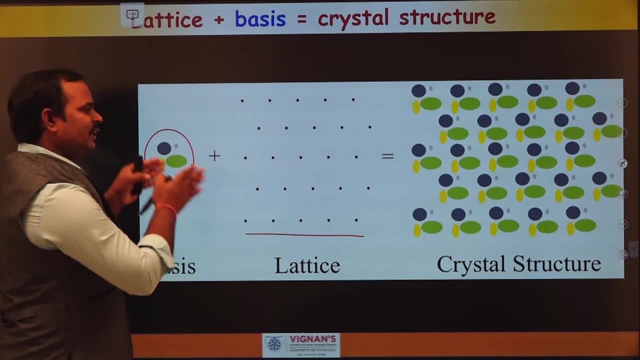 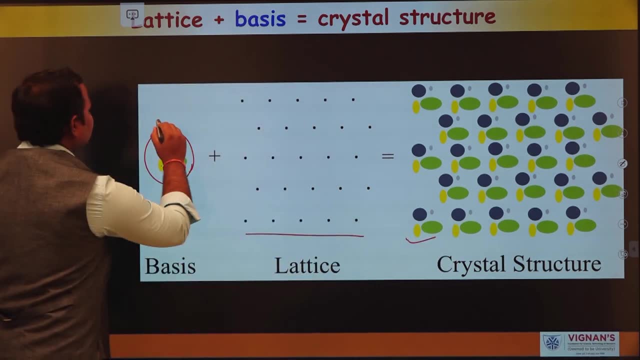 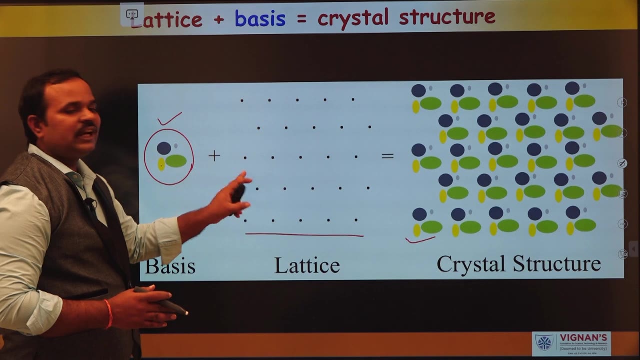 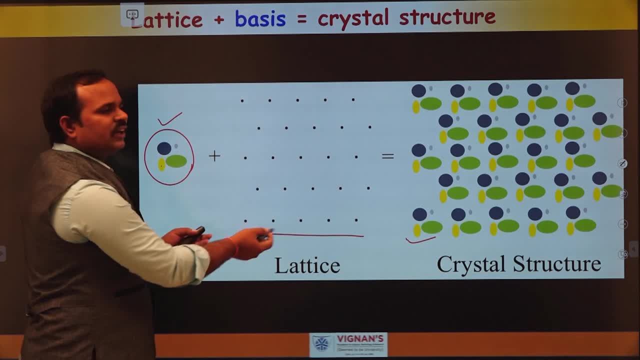 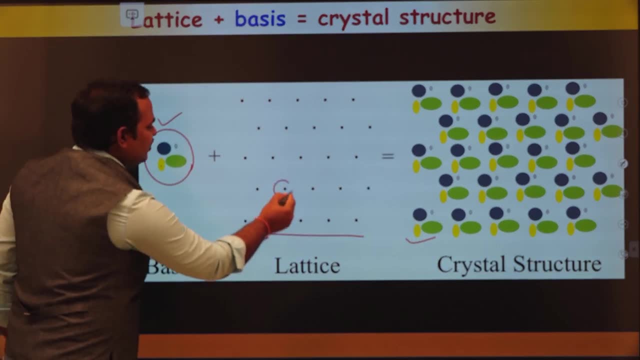 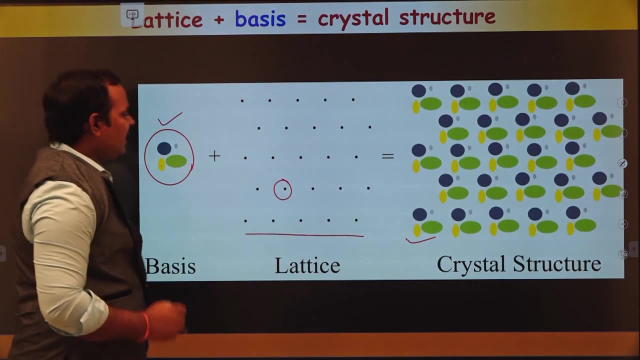 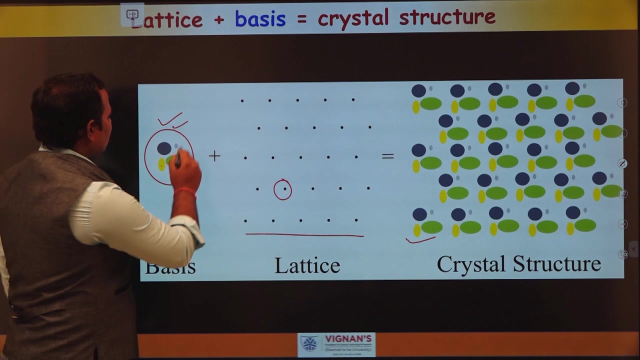 This is a real crystal, but this is a geometrical concept of this real crystal, where the points are arranged in the space such that the environment about each and every point is identical. That is the reason why we get a uniform crystal structure And the basis is a structural unit where it could be one atom or a group of atoms. 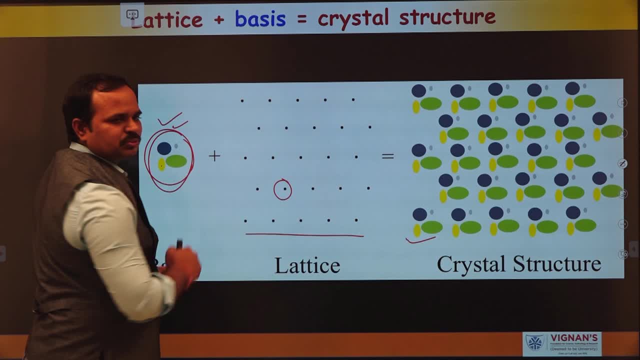 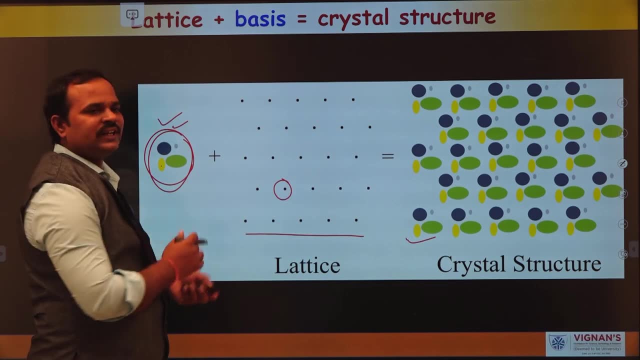 Now these group of atoms must be replaced at each and every lattice point to get a total crystal structure. So this is how we get a total crystal structure. We can visualize any crystal structure in the universe. So in summarizing, so a lattice is: 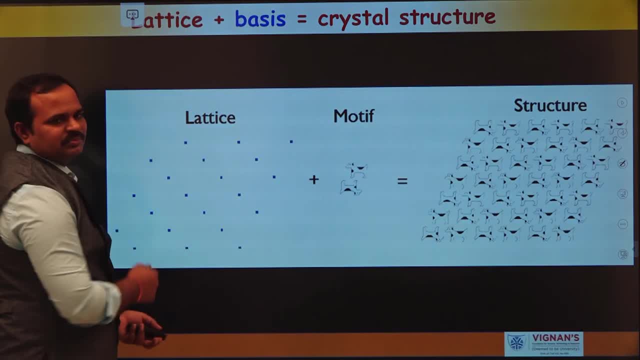 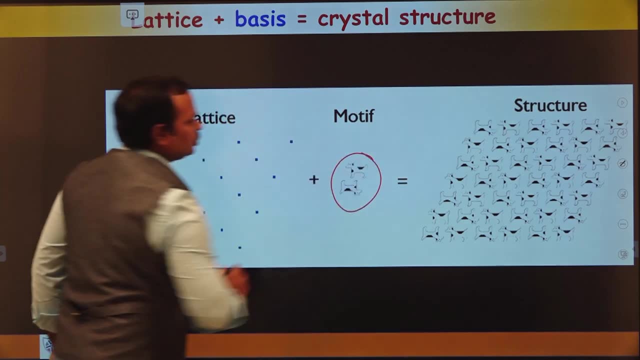 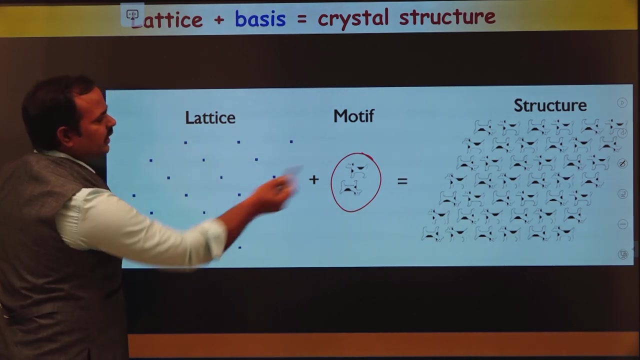 a lattice. This is a lattice constructed by using some translational vector. Here this is a basis. Here the basis is two dogs, small dogs, which are inverted. Now the basis. you need to keep at each and every lattice point to get total crystal. 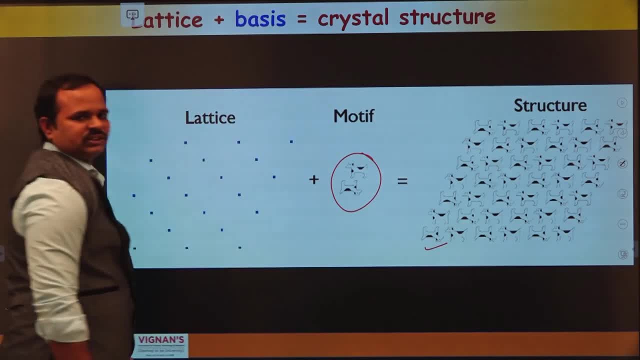 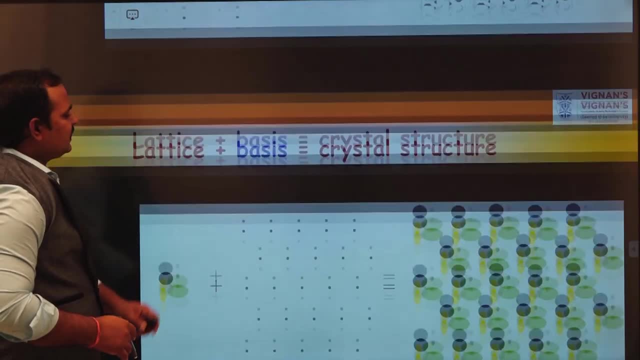 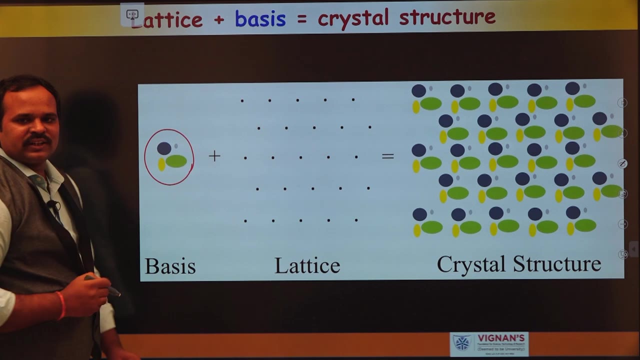 structure. This is how you get a total crystal structure. In place of this, you can have two different atoms which are inverted. The another example is- this is one You can see here. this is the basis atoms. There are four atoms are there and. 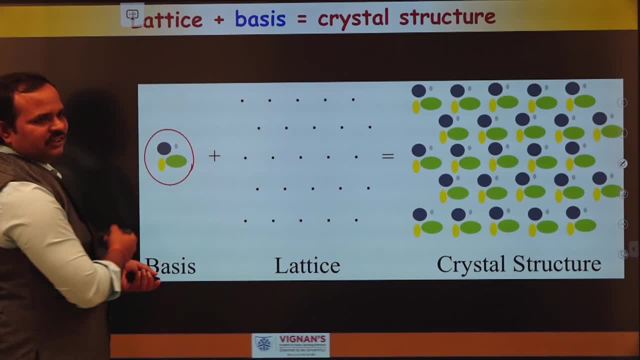 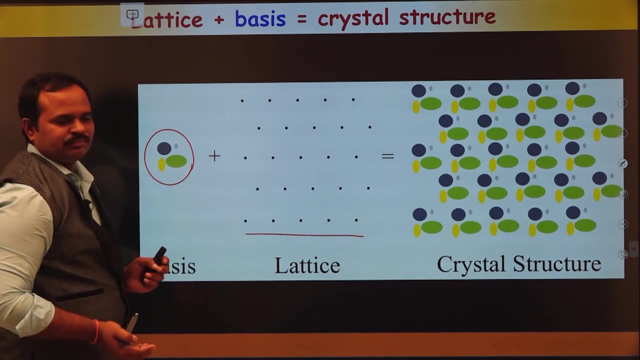 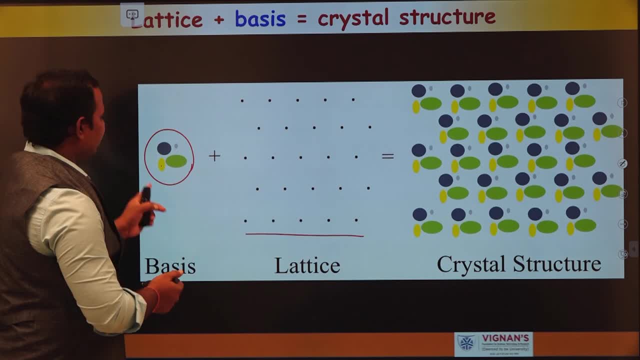 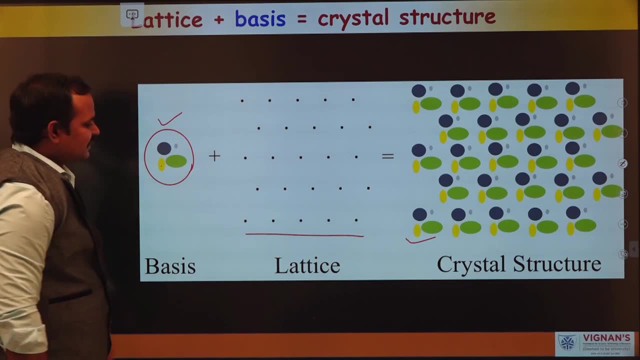 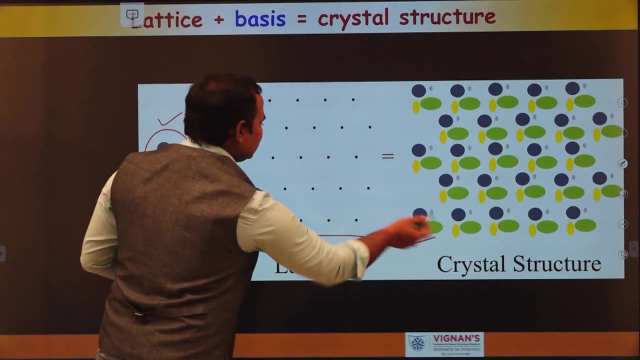 orientation and chemical uniformity is not changing, Then we get total crystal structure corresponding to these four atoms. So that means the lattice is a geometrical concept of a real crystal. This is a real crystal. but this is a geometrical concept of this real crystal where the points are arranged in the 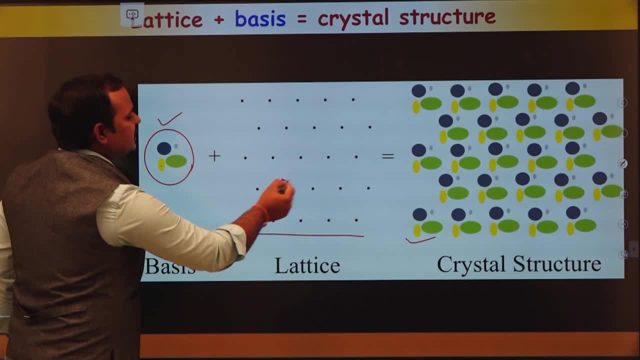 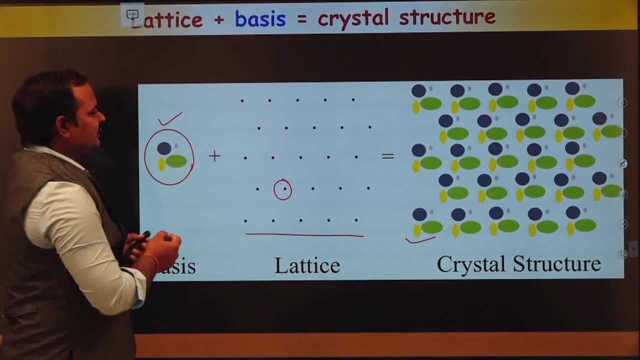 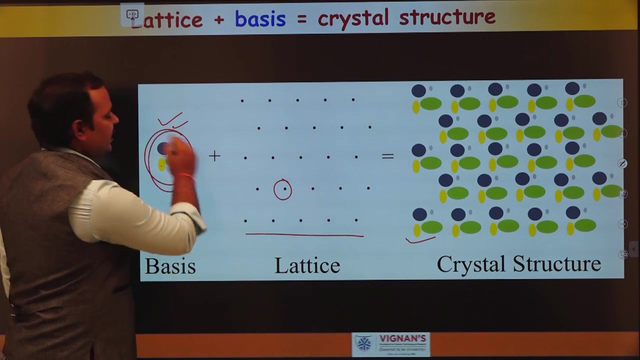 space such that the environment about each and every point is identical. That is the reason why we get a uniform crystal structure And the basis is a structural unit where it could be one atom or a group of atom. Now this group of atoms must be replaced at each and every lattice point to get a total crystal. 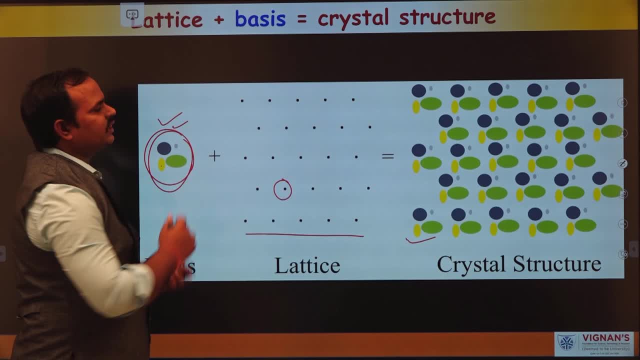 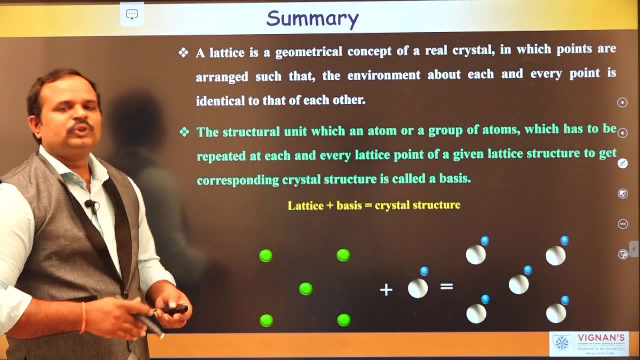 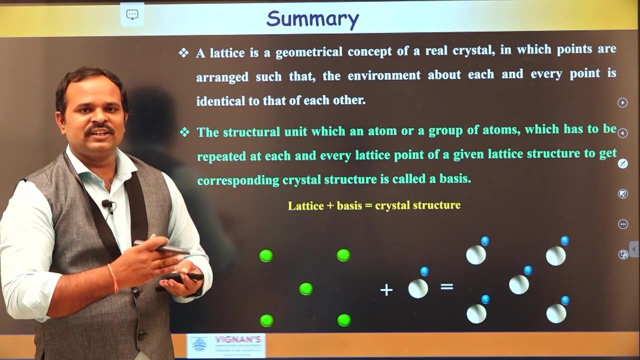 structure. So this is how we get a total crystal structure. We can visualize any crystal structure in the universe. So, in summarizing, so, a lattice is a geometrical concept of real crystal in which the points are arranged in the space such that the environment about each and every point is identical.